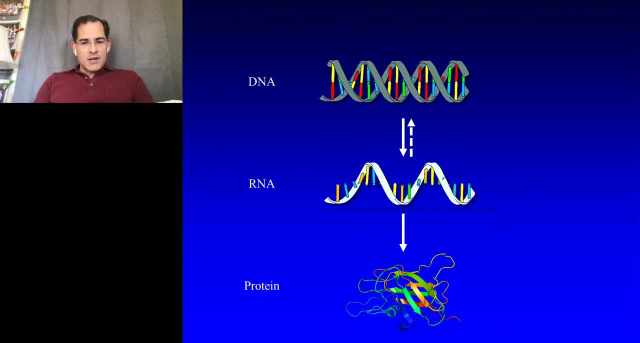 So if we take a step back and consider the basic biology that underlies all biological function, we can see that, of course, DNA encodes all the genetic information on the planet, and this information can then be transcribed within organisms into RNA. 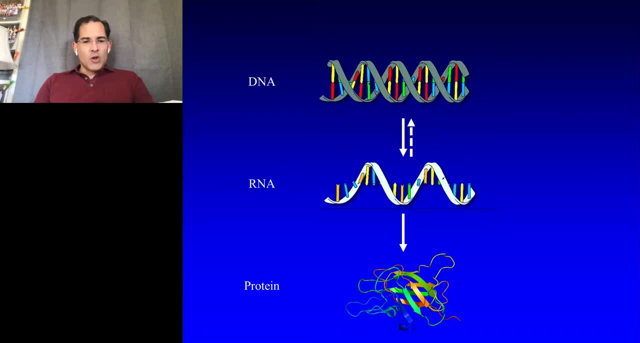 and then that in turn becomes translated into a protein, And this flow of information from DNA to RNA, to protein, of course, is called the central dogma of biology. From the point of view of somebody who's trying to develop a therapy, we can view each one of these levels as a potential drug target. 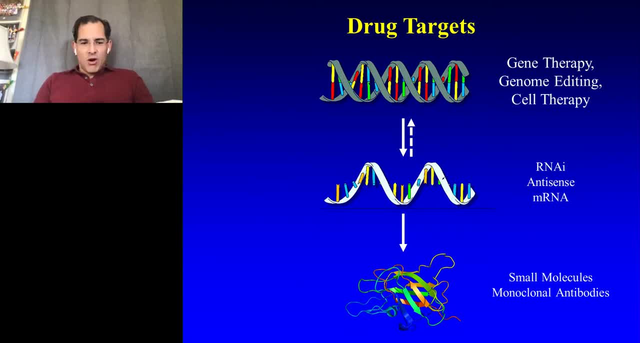 So the majority of pharmaceuticals that are currently in use target at the level of proteins. Small molecules float around, typically bind hydrophobic pockets such as the active side of an enzyme and inhibit or alter the function of that enzyme. Monoclonal antibodies float around. 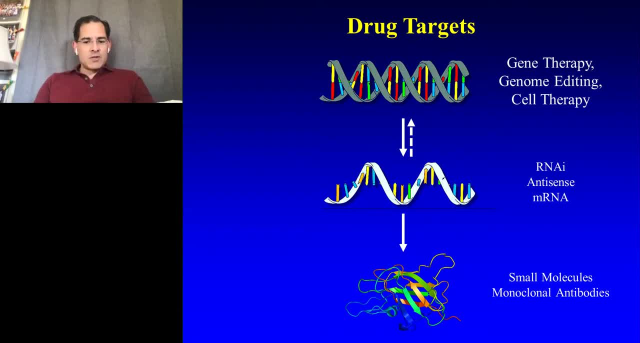 and bind to protein targets floating on the outside of the cell, such as a growth factor or receptor. So if we move back one level, you can begin to develop therapies that work at the level of RNA inside of the cell. So these include RNA interference or antisense RNAs whose goals 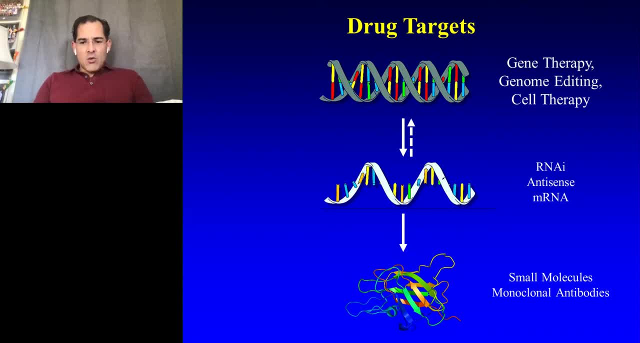 are to knock down the production of proteins from RNA or messenger. RNA itself can actually be a therapeutic molecule, But, moving back one further level at the level of DNA, this has really been the focus of my entire career. So, gene therapies, the delivery of new genetic 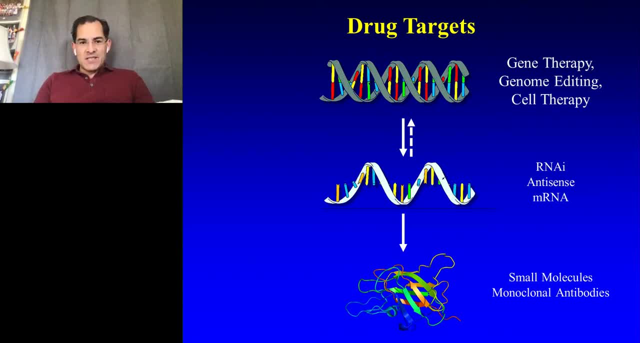 to a cell genome, editing, the changing or the editing of existing genetic information inside of a cell or cell. therapies or stem cell therapies, where the goal is to deliver an entirely new. so the power of targeting dna to be able to affect a therapeutic outcome is that the fact that dna, unlike small molecules or proteins, are actually 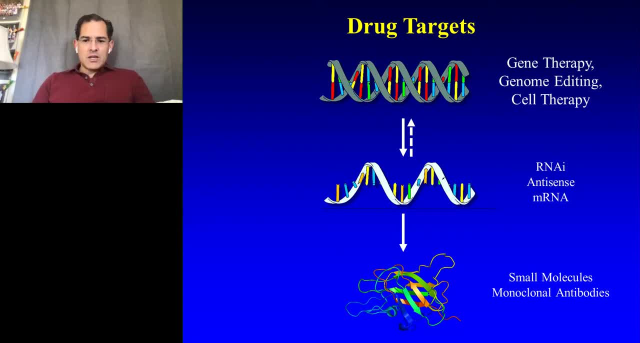 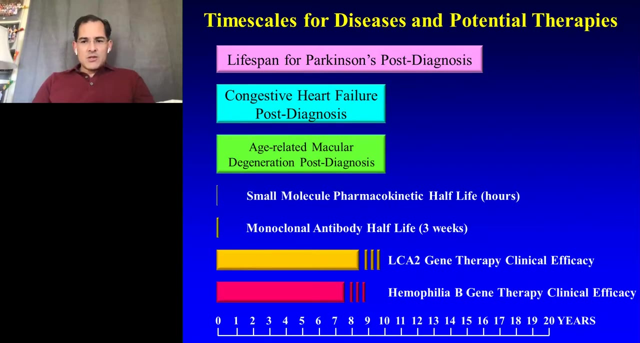 tissue, so new dna to a cell or tissue that can potentially persist for the life of a patient, which raises the possibility of single administration long-term patient benefit. so just to illustrate this idea we have here the on the x-axis the number of years that an individual is affected by a particular condition. so typically post-diagnosis parkinson's patients. 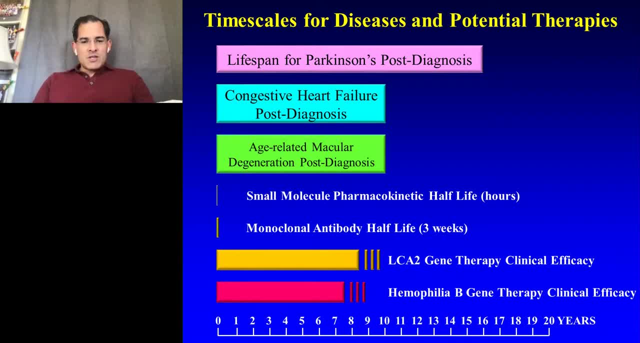 on the order of another 16 years or so. so congestive heart failure- between diagnosis, ultimately when a patient passes away due to chf- is on the order of 10 years. age-related macular degeneration itself is an addition. it robs people of their vision, but typically does so. 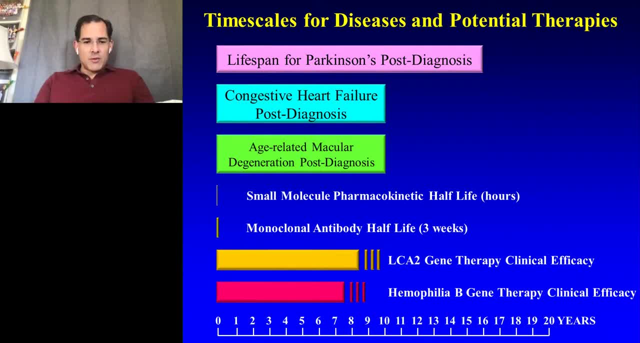 towards the lifespan, so they typically die of other causes after around 10 years of diagnosis of amd. so if we consider or compare these to the lifetimes, the pharmacokinetic half-lives, if therapeutic modalities that are being developed to be able to treat these conditions, we have a small molecule with 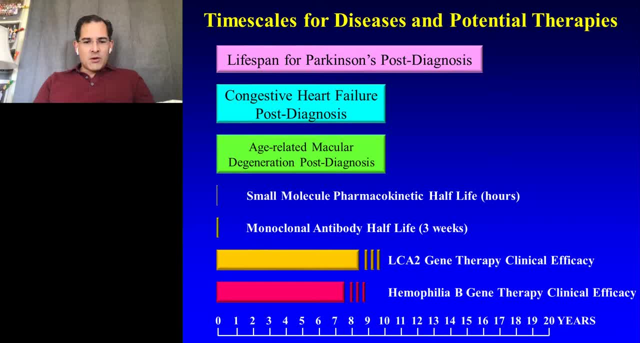 a pharmacokinetic half-life on the on the order of hours. monoclonal antibodies: last days to several weeks. however, dna in the form of a gene therapy can potentially last years or even decades. so here are a couple of examples of gene therapies, one of which i'll be discussing in more detail. 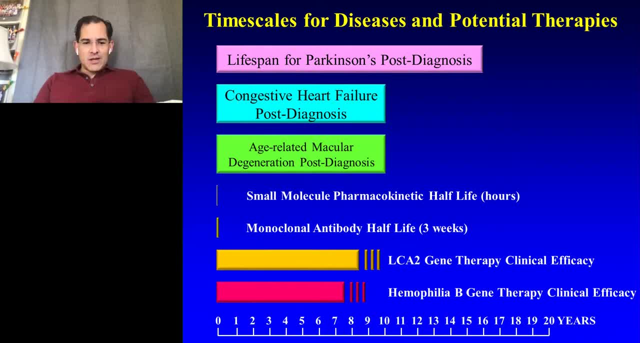 where a single administration back in the 2000s led to, in some cases, over a decade of therapy and in some cases over the course of a decade or even decades. so this is an example of a gene therapy that was developed in the early 2000s and was developed in the early 2000s by a group of 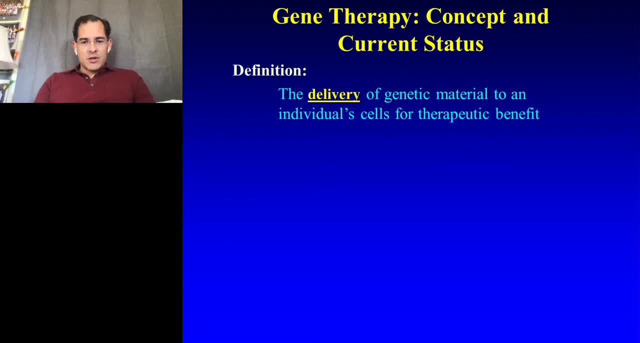 physicians who were interested in the therapeutic benefit from the patients who were still enjoying the fact that they received this gene therapy many years ago. so let's all get on the same page and actually define what gene therapy is. is the delivery of genetic material to the cells of an 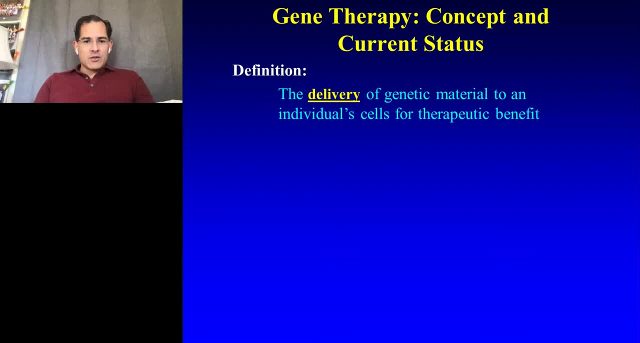 individual patient for therapeutic benefit, and so, while this idea was originally proposed back in the 1960s, we've had to wait for 50 years in order for it to begin to come to fruition, and the reason for this is that gene therapy is a very large molecule. it's difficult to get it past the cell. 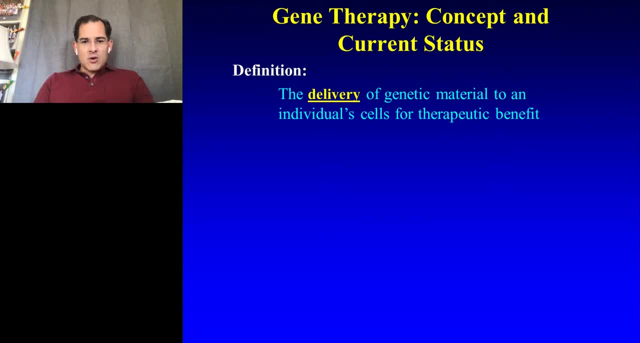 membrane and into the nucleus of a cell and in addition, on its own floating around in the blood stream. dna is not particularly stable. it's degraded by nucleases that are present, so it's been hard to be able to develop delivery vehicles or vectors that can carry dna inside of enough. 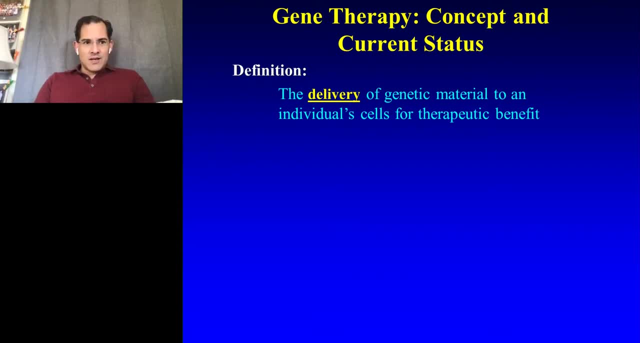 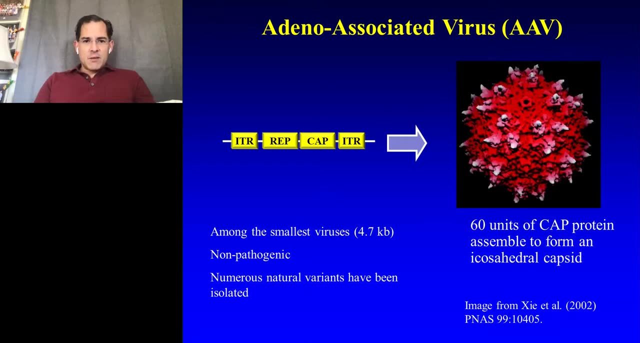 cells within it to to begin to move the meat, the needle, on treating a disease. so the way that this has been achieved in the field increasingly over the past decade is that gene therapy has been around for a couple of decades, is that people have been identifying viruses very effective? 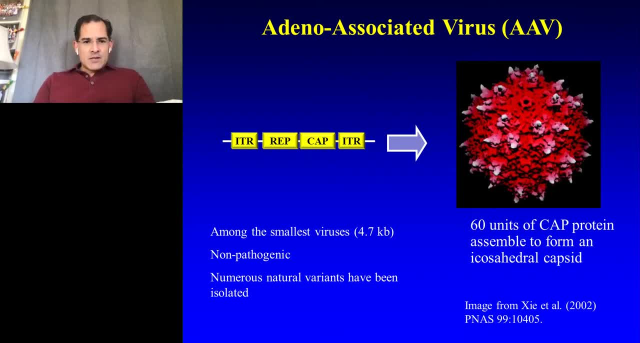 viruses that can carry dna inside of cells, so aav, or adeno associated virus, is a particularly interesting one. it has risen to be the most promising virus within the field of gene therapy for a couple of reasons, first and foremost- which, of course, is a major factor to discuss today. 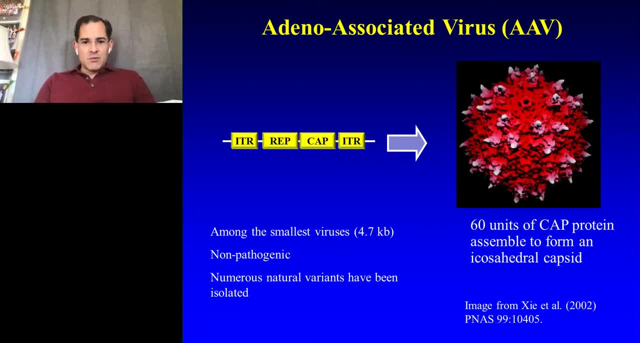 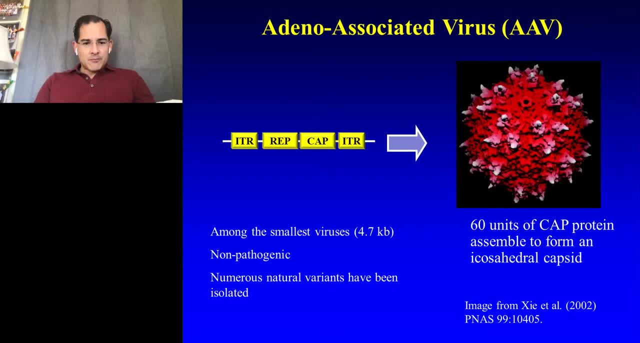 it's a harmless, non-symptomatic virus. in addition, it's among the smallest of viruses, so if you take a look at its genome structure here, it has two genes called rep and cap, and the rep encodes some enzymes that mediate the replication of the viral dna. the cap has really been the focus of about. 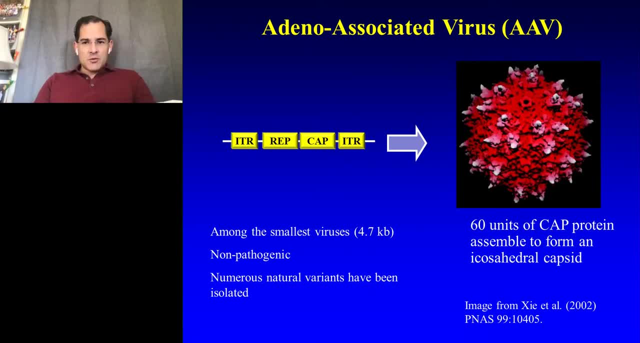 half of my career, because the cap encodes some non-structural pro- sorry, some structural- proteins, around 60 copies of which self-assemble to form this particle here on the right hand side and the particle as you can see. on the top side of it there's a black circle. it contains a pore. 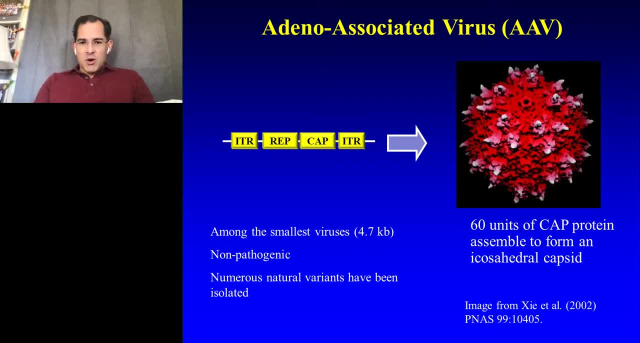 at what you call the five-fold axis of symmetry, and once this particle is assembled, one copy of the viral dna will snake its way inside of that pore to be able to load the virus with its own genome- only around 4.7 kb in size, and the particle is around 26 nanometers in dimension. 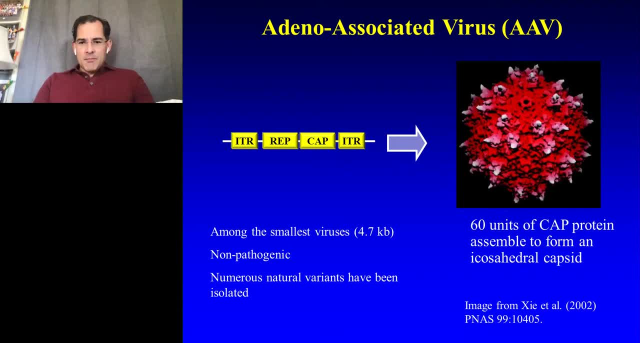 importantly, a number of variants- well over a hundred- have been identified and contain a lot of sequence variations in the amino acid compositions on the surface of the virus. so those white peaks, for example, that you see emanating from the core of that viral particle, and these changes in the surface. 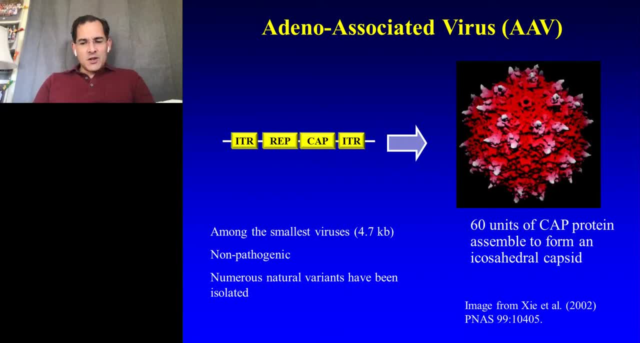 composition of the virus have been correlated with changes in the delivery of the pathway and the device, by distribution and the cell preferences of the virus, which raises the possibility that by engineering the surface of the virus you can actually create highly efficient and breeds basic Вотto effects in certain areas of reaches in severaligeners and, For example, 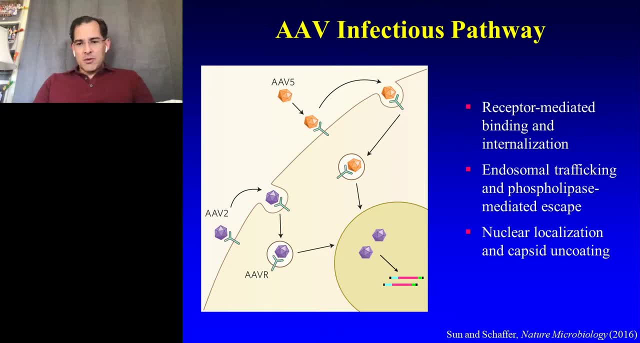 My prediction for this study is that the receptor image unidirectional cell brain can actually explore multiple olhos out of a cell. basically taking on Verodia is such that, by creating an analogical resonance of the pole, the virus is actually inspiring and the viral protein that enables it to sneak its way past that lipid bilayer that surrounds it. 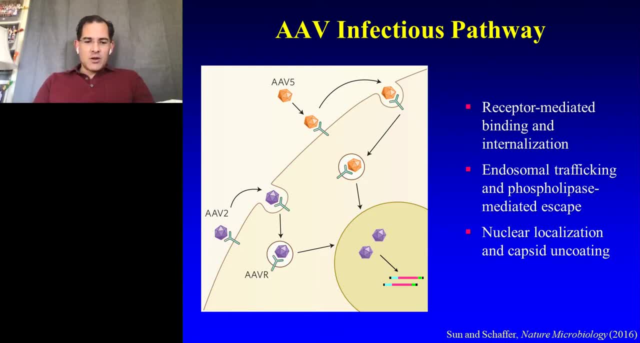 and then eventually finds its way into the nucleus, uncoats the viral capsid and releases the viral DNA, which can then go on to carry out subsequent steps in the viral life cycle. And the way you turn this into a therapeutic is: you quite simply take 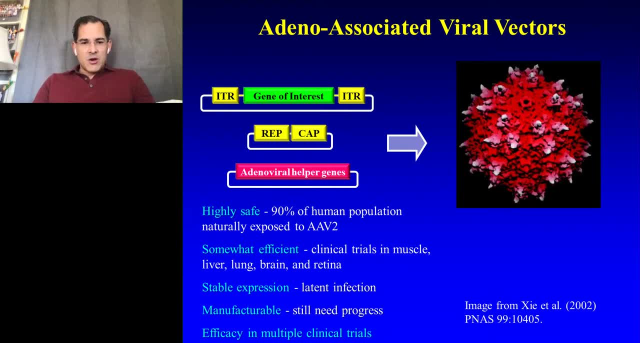 the rep and cap genes, delete them from the viral genome, place them onto a subpiece of DNA, and this results in two outcomes that are advantageous. One is that it liberates space for the insertion of a gene of interest between those flanking sequences, those ITRs, and, as a 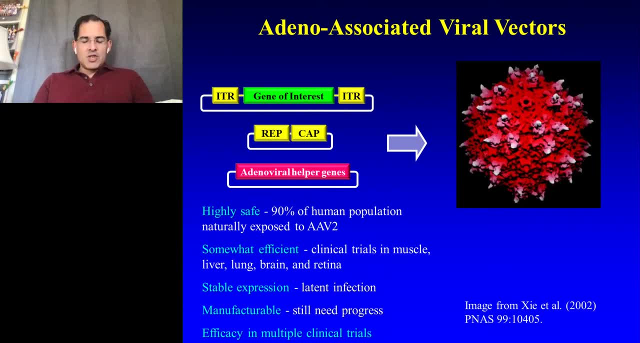 result, when that viral particle on the right-hand side is assembled, that gene of interest becomes internalized into the viral particle and you leave your virus then with a piece of medicinal or therapeutic DNA to treat a disease. In addition, as a result of the fact that the rep and the cap, 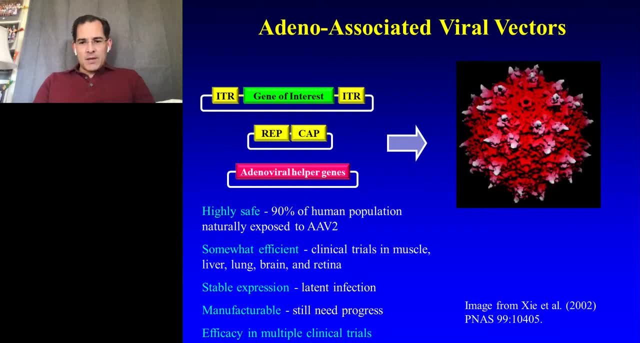 no longer make an incisor. the rep and the cap no longer make an incisor. the rep and the cap no longer make an incisor of the virus. this is no longer a replication-competent virus. It simply deposits the gene of interest into the nucleus of a target cell, and that DNA can then persist for long. 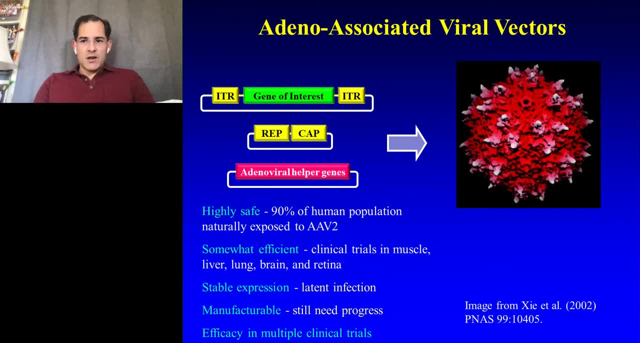 periods of time and be able to produce a therapeutic product, such as an RNA molecule or a protein molecule, to treat a disease. So this resulting recombinant virus has a number of advantageous properties. It's very safe. Like I mentioned, 90% of the human population has already. 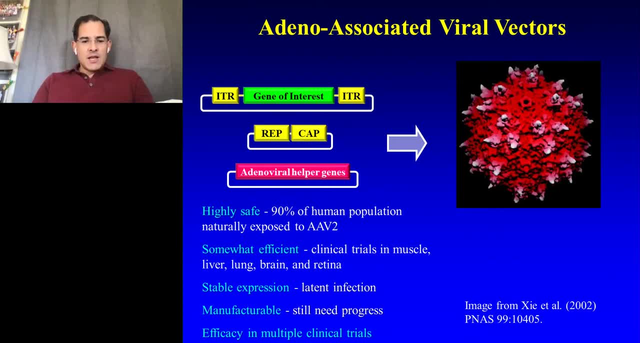 been exposed to one or more natural variants of AAV. It's somewhat efficient. The natural variants are and have been used in over 200 human clinical trials involving delivery to muscle, liver, lung, brain and retina. The product of that genome after delivery is very stable. It can persist. 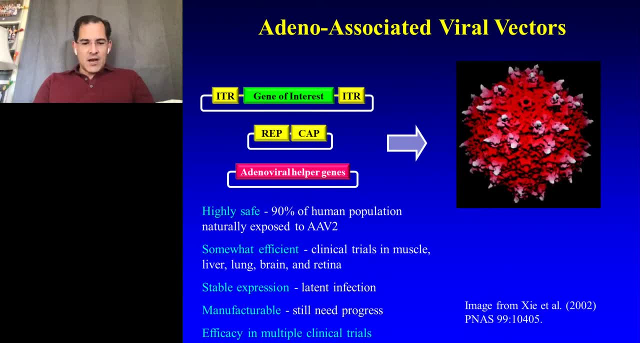 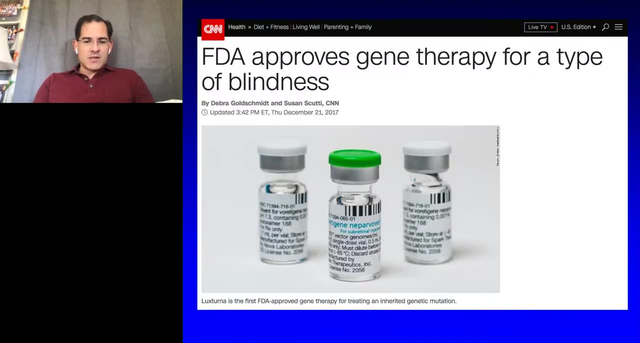 at least in non-dividing cells, for years or a decade and counting, And it's possible to manufacture these at high yields. And as a result of all these properties, the virus is enjoying success, with an increasing number of human clinical trials, resulting, for example, back in 2017, in the 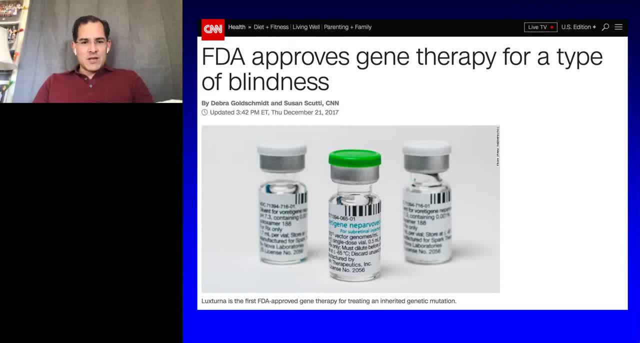 first FDA approval of a gene therapy for a rare disease, And this therapy was based upon an AAV virus and it was to treat a blinding condition called Leber's congenital amaurosis type 2.. So this is currently being developed and commercialized and sold by Roche Therapeutics. 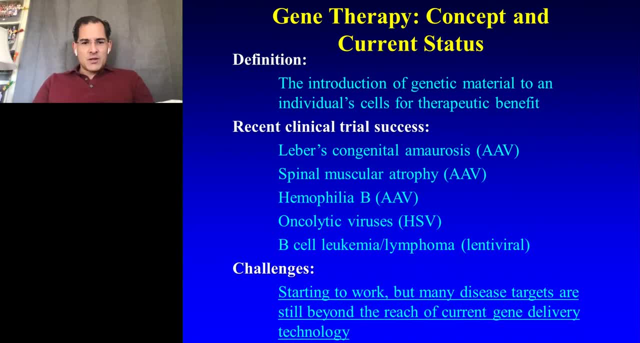 So we've seen an increasing number of successes within clinical trials: that LCA disease that there was an FDA approval for in 2017.. We've seen an improvement in the gene therapy for the smallpox and left blood cells. We've seen an improvement in the gene therapy for spina muscular atrophy from Novartis. 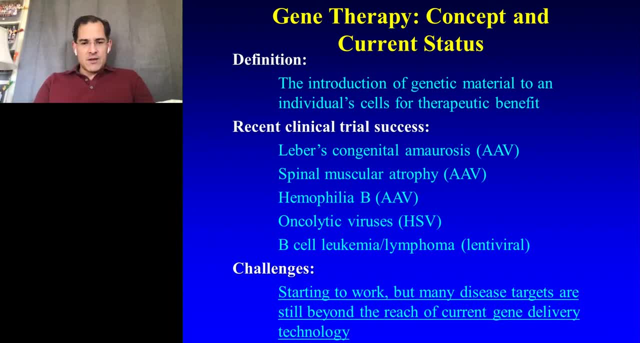 to be able to treat a rare condition which results in fatality and progressive paralysis and fatality of young boys. Hemophilia B has advanced to a pivotal trial, a phase three clinical trial, and shown strong promise. Hemophilia A is not that much further behind. 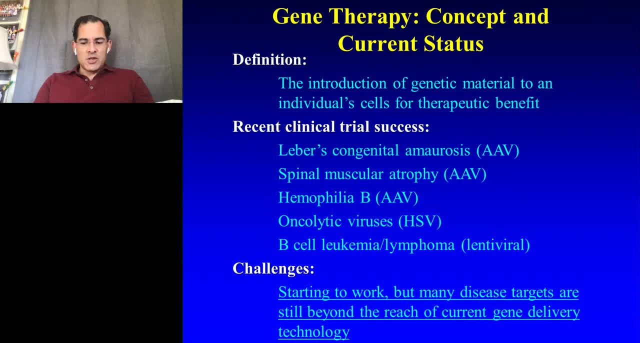 And we have a long list of successes and- well, not that long yet, but increasingly field. However, these successes have resulted in some pretty savvy clinicians who've identified diseases where the properties are just good in genetic efficacy, But even so, these viruses. 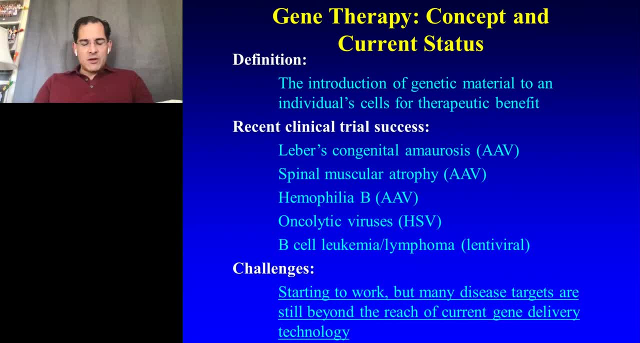 were not designed as pharmaceutical gene delivery vehicles And, as a result, these investigators have had to really brute force the delivery, had to use very, very high dosages of virus or have had to use invasive routes of administration to place the virus right next to the target. 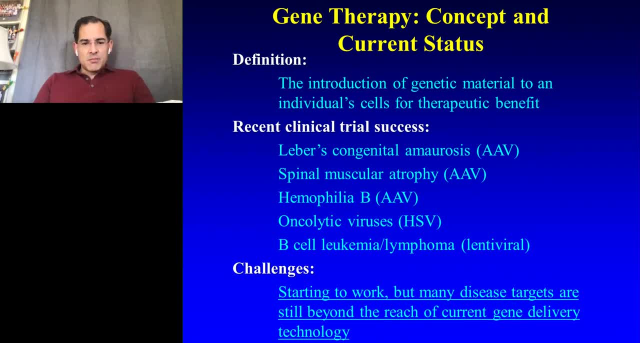 cell, And the field knows that, to be able to build upon these initial successes and extend them to the majority of human diseases, we quite simply need better viruses. So, in other words, gene therapy is starting to work, but many diseases are still beyond the capabilities. 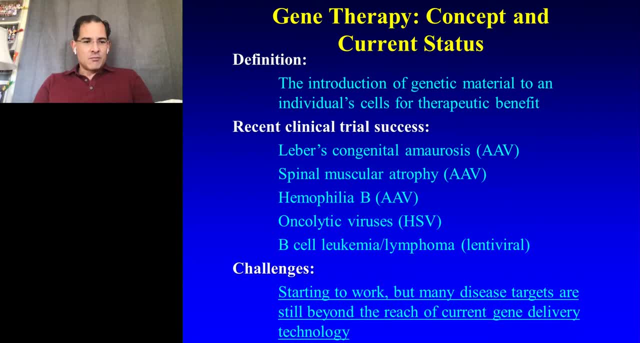 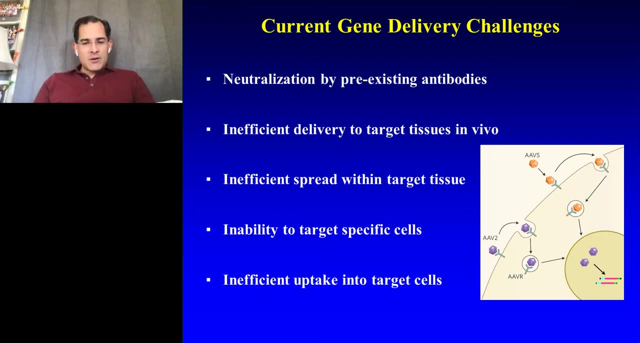 of current delivery technologies and we need new AAVs. So thank you. So what are some of the existing challenges with AAVs? The first one I've indirectly alluded to already, which is the fact that 90% of us have already been exposed to one or more. 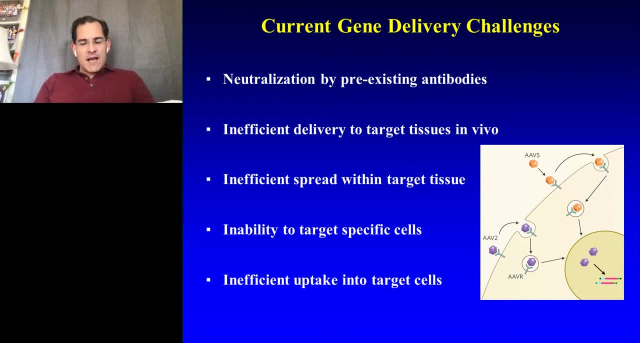 AAV variants And, as a result, we've been accidentally vaccinated against the virus and high concentrations of antibodies that will neutralize natural versions of AAV, And so that's a significant barrier within the field. It's, in fact, the most common reason. 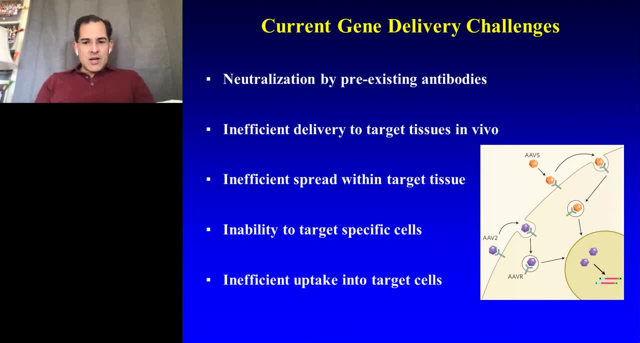 that patients are turned away from clinical trials. In addition, after the virus potentially makes it past those antibodies, it inefficiently distributes to most target tissues inside the body. It tends to go very well to the liver, but not as well to many other tissues. There's inefficient spread. 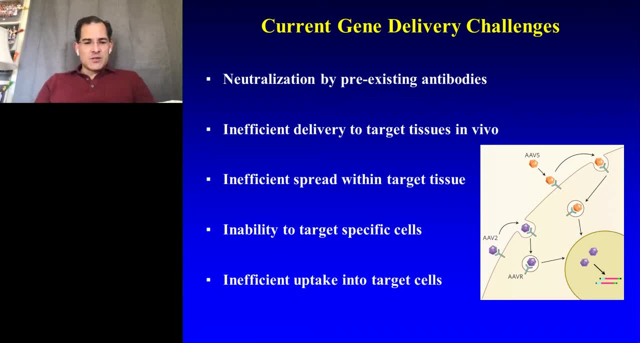 within those tissues. Once the virus is able to reach the surface, it can't penetrate deep inside of that tissue. If it reaches near the target cells, it has the ability right now to target delivery to some cell types, but not others, within that tissue And even 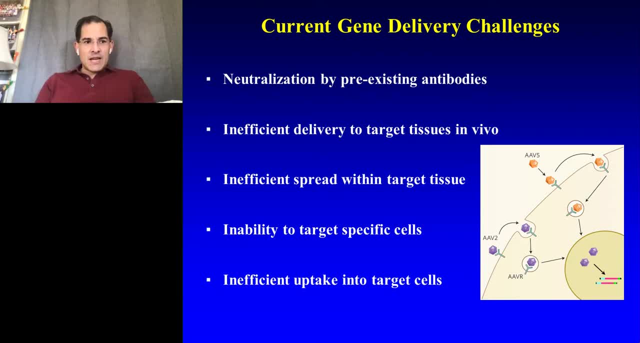 if it reaches the surface of an intended target cell, it's often taken out very poorly by that cell. So these are, after all, respiratory viruses and it's a lot to ask of them to be able to very efficiently infect other target cell types such as a neuron or a cardiomyocyte. 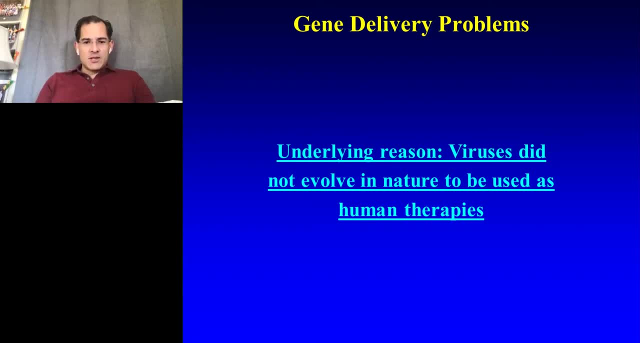 So all these shortcomings arose from a very simple fact, which is that nature never evolved viruses for our convenience to use as medicines, And so, around 20 years ago, we developed a hypothesis that, if we'd like to improve the properties of these viruses for therapy, we 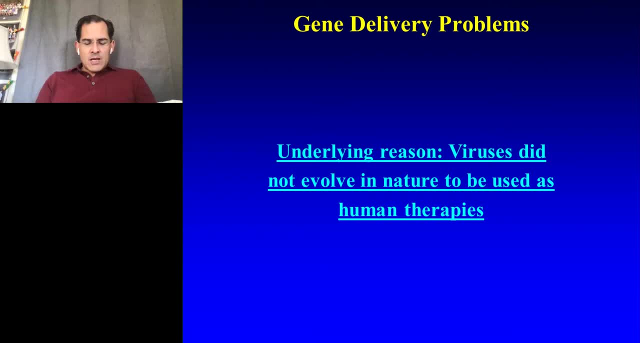 need to re-evolve them or re-engineer them at the molecular level. The toolkit or the methodology that was emerging in the field, that we saw at PROMIS in enabling us to do this, was the product of an investigator by the name of Frances Arnold. 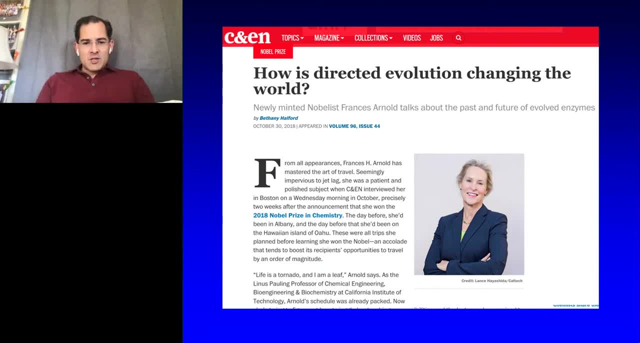 She actually graduated from Berkeley back in the 80s and since then she's been a professor at Caltech And she won the Nobel Prize in Chemistry in 2018 for the concept of using evolution as a tool to design novel function into biomolecules. 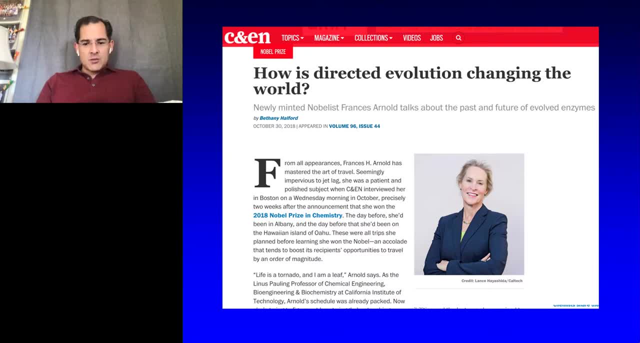 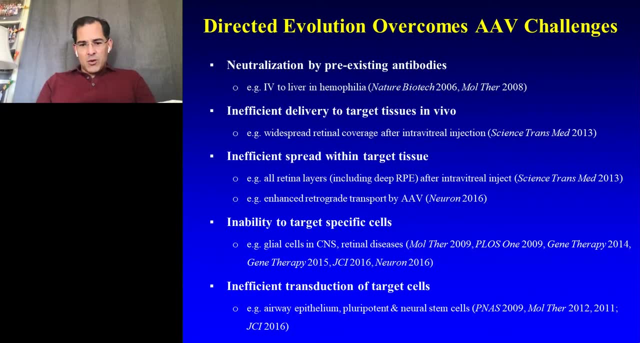 So she did this specifically with industrial enzymes and we became the first to do it with viruses like AAV. So this approach about directed evolution- and I'll explain how it works in just a second- we've been conducting it the past 20 years with AAV and we have multiple examples in 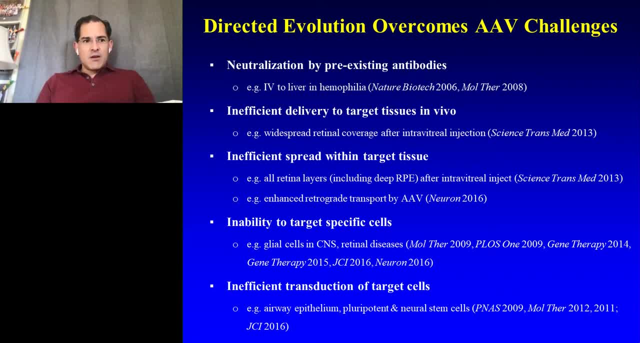 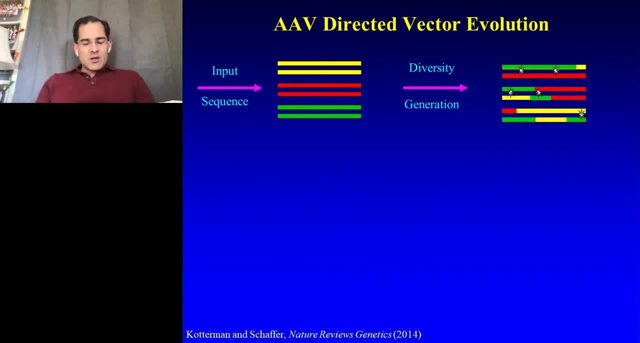 which we've used this approach to be able to create new AAVs that have overcome some of these barriers I talked to you about before, with a variety of cell and tissue targets. So the way that this technology works is it's based upon evolution, and evolution has two. 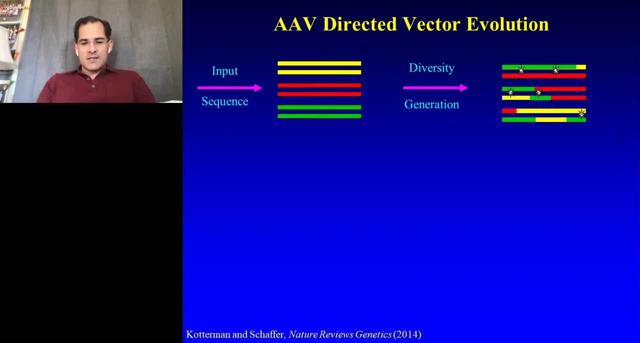 basic steps. The first is to create a gene pool and the second is to select the fittest. So as a gene pool, we take several natural versions of this virus and we perform a number of steps to genetically diversify them, And specifically I'm not going 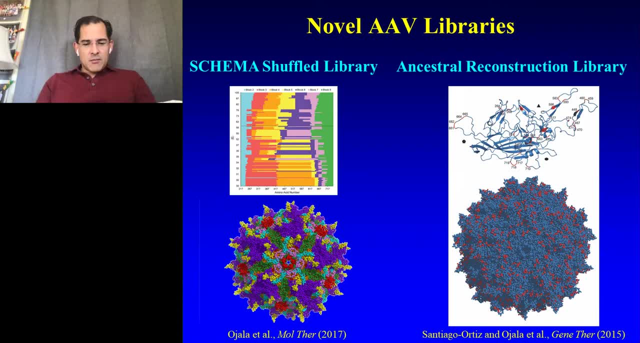 to go into this in great detail, but we've created some libraries in which we've generated chimeras of several of these parent viruses and generated new variants that contain pieces of individual parents. We've used bioinformatics and computational approaches to reconstruct family trees of AAVs and began to predict sequences of these viruses that may have. 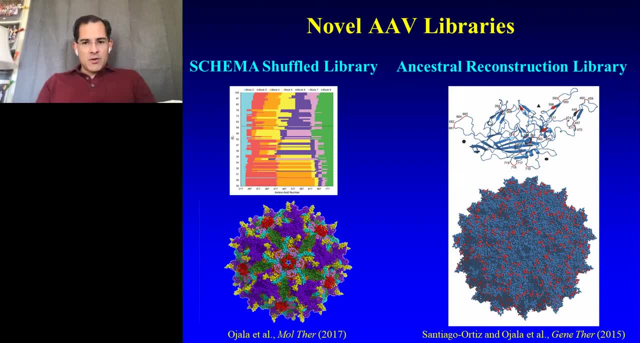 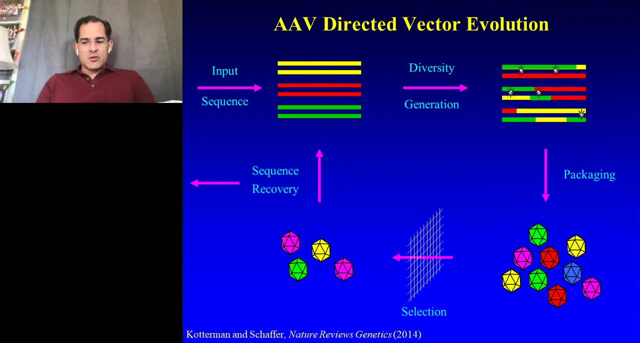 existed a long time ago and built libraries around those- a process known as ancestral reconstruction- And in fact we have those two libraries and 35 others that we've utilized to introduce diversity into that viral co-protein in a variety of different ways. So that's the gene pool. 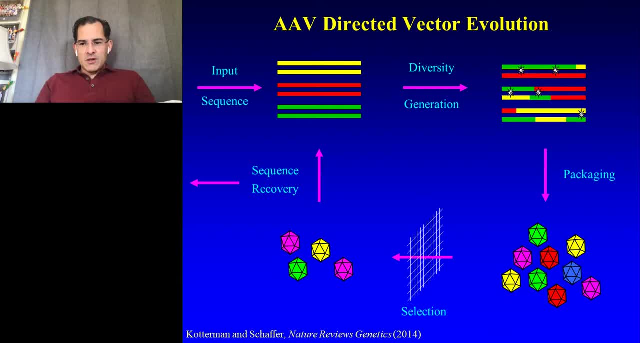 where we then package these into libraries of particles where every single variant or every single particle is composed of a variant protein. shell Variant capsid contains inside of it the DNA that encodes that capsid. So we'll then, as the second step, play Darwin, select the fittest, and I'll describe to you some selections. And by spinning, 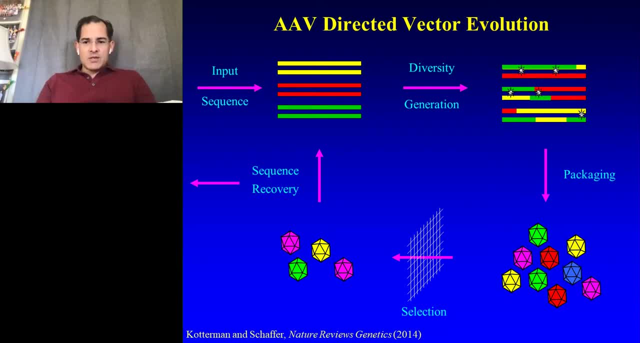 around this loop. iteratively. we can end up evolving or selecting variants that have desirable properties And, at any point along the way, pop open the particles and sequence the genomes to recover the information, the sequences or composition of those capsids that mediated the efficient gene delivery or the efficient 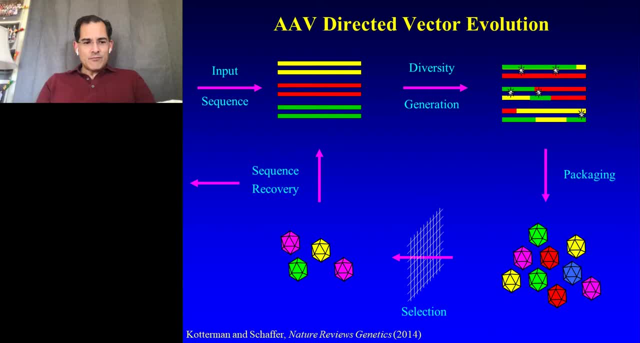 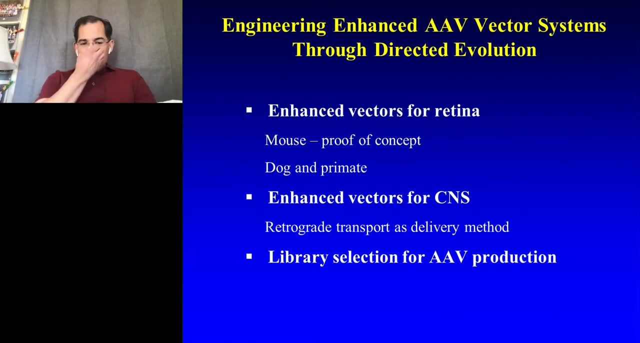 targeting to a given specific tissue, And once we have those new engineered capsids, we can then begin to utilize them to deliver DNA medicines. So just to outline, today I'm going to show you a couple of topics that we've been working on. 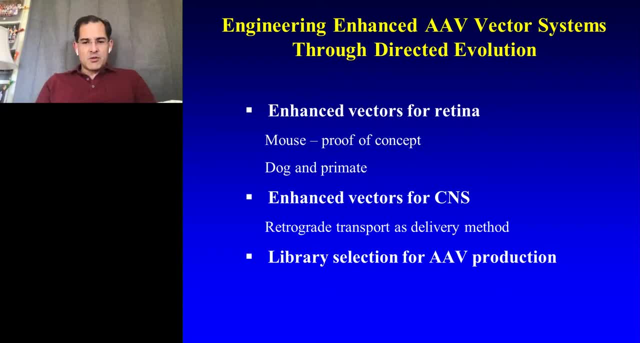 One is engineering AAVs for the retina to be able to treat blinding conditions, Another is for the central nervous system, And then I'm going to switch gears a little bit afterwards and talking about our efforts towards using this approach to be able to solve problems in process engineering. 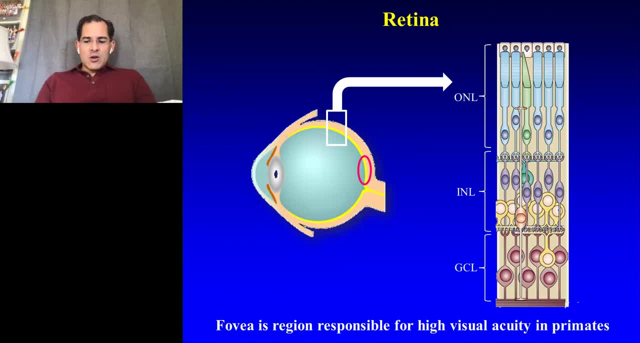 So let's get started. So we're going to start with the first one, which is the gene therapy for AAVs. So, as I mentioned to you, the very first FDA approved gene therapy for rare disease involved in AAV, for treatment in the retina And this is the structure of your eye. 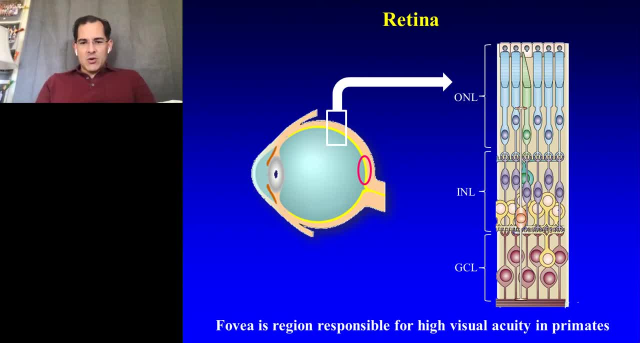 At the back of the eye you have a number of layers of neurons that are painted onto that surface area, And all the way at the back is the so-called ONL or outer nuclear layer, and this contains the photoreceptor neurons, cells that sense photons. 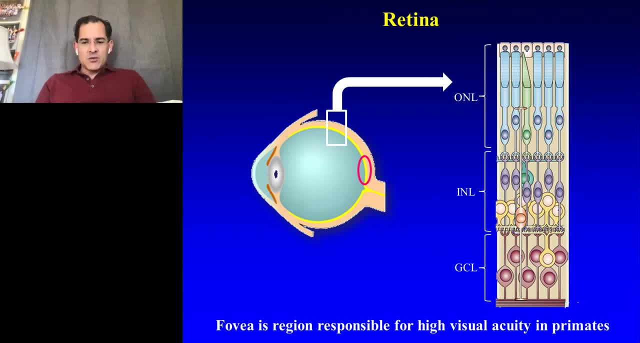 So once an action potential and communicates that information to various interneurons in the INL inter-nuclear layer and GCL, the ganglion cell layer, And these GCL neurons will then send information along their axons through that white line that lies at the or sorry. 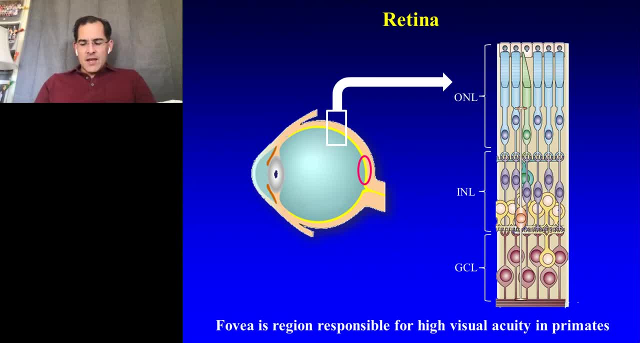 yellow line at the back of the eye which is the optic nerve, And the eye then communicates that information to the brain for further processing. So the place you would like to be able to. oh, one final point I'd like to make is that in the back of the eye, in the center, there's a region called the fovea. 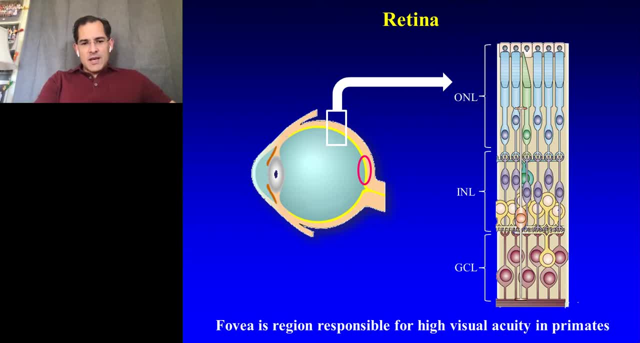 that contains a high concentration of cone photoreceptors, And this is what's responsible for high visual acuity. So if you're reading a page and your eye scans back and forth, what your eye is doing is keeping the light from a page focused in on the fovea. 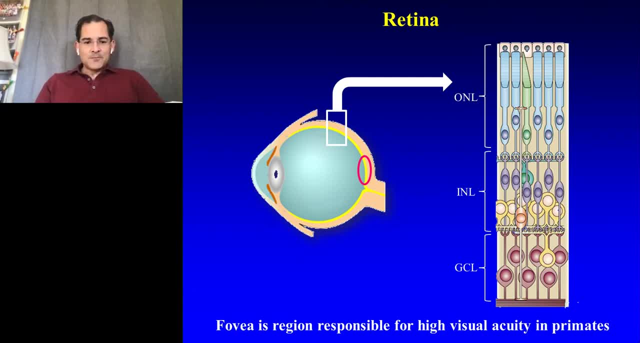 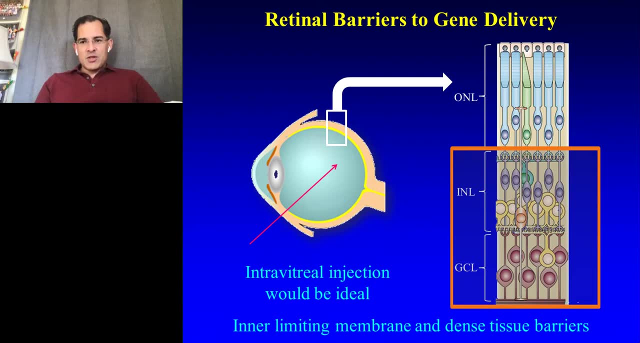 because you need that high acuity vision in order to read the page. So this is an important region of the retinas to protect. So, unfortunately, mutations in over 200 different genes can result in the death of photoreceptors. So this is an important region of the retinas to protect. So, unfortunately, mutations in over 200 different genes can result in the death of photoreceptors. 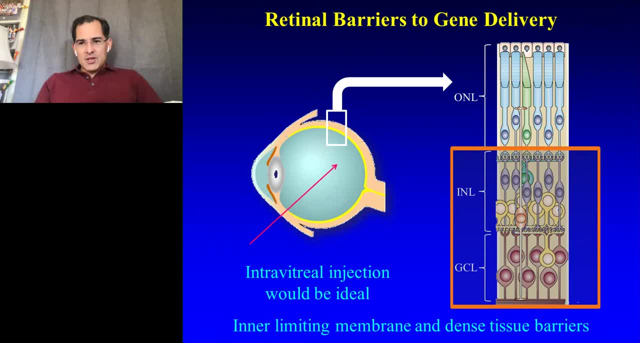 brace. so the place you would like to deliver a drug to be able to treat these conditions is through the vitreous of the eye, which is this fluid or gel like substance in the inside of the eye, because if you can do an injection there it's. 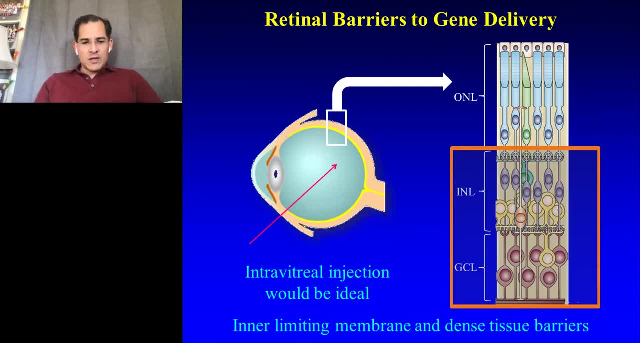 very simple. it takes around four seconds, local anesthesia only only, And this gives your drug the opportunity to be able to diffuse throughout the eye and to come into contact with the full surface area of the retina and therefore protect the majority of cells inside the retina. And in fact, this intervitreal injection is conducted several 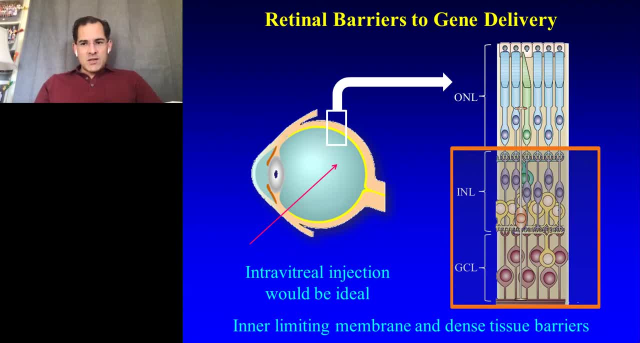 million times a year in the United States to deliver protein drugs produced by Genentech and Regeneron to be able to treat age-related macular degeneration. So, unfortunately, unfortunately, the cells of the INL and the GCL represent a barrier where you would like. 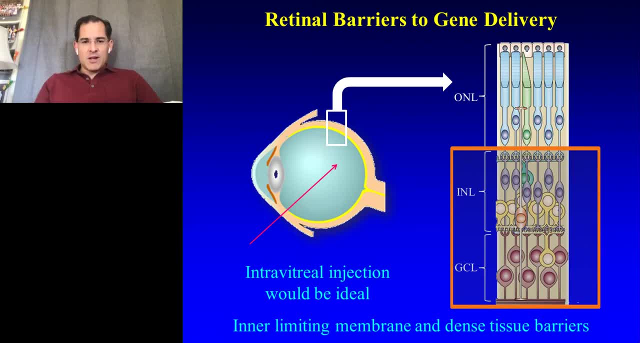 your AAV to deliver the DNA medicine to the photoreceptor neurons. That's the target for the therapy, But unfortunately no natural version of AAV can actually distribute or transport through the several hundred microns of dense tissue it would take to be able to make the trip from the 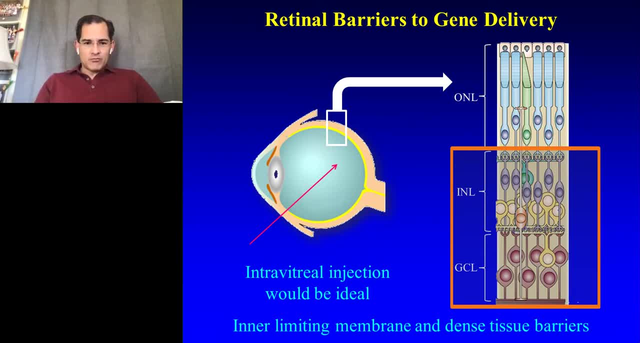 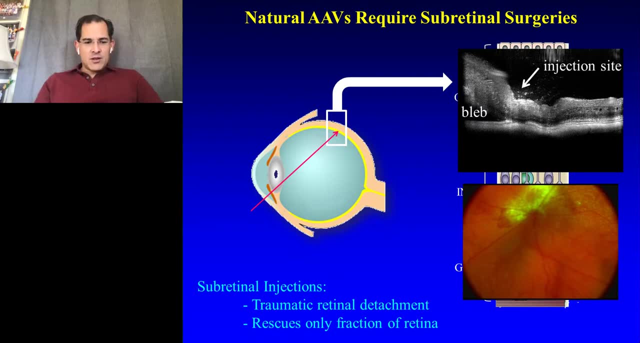 vitreous fluid all the way back to the adrenuclear layer. So, as a result, natural versions of AAV have to be injected right next to that target cell. So in that FDA-approved product, for example, which uses AAV2, natural serotype 2 for AAV, they have had to take the needle, actually puncture it. 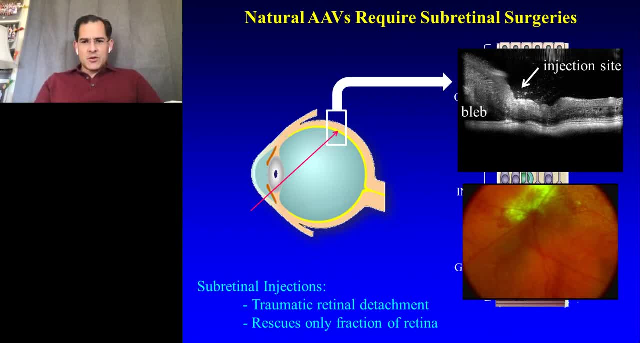 through the retina and inject fluid between the adrenuclear layer and the underlying retinal pigment epithelium, And this is problematic for a couple of reasons. So first of all, it detaches the retina And at the injection site this retinal detachment can actually cause some 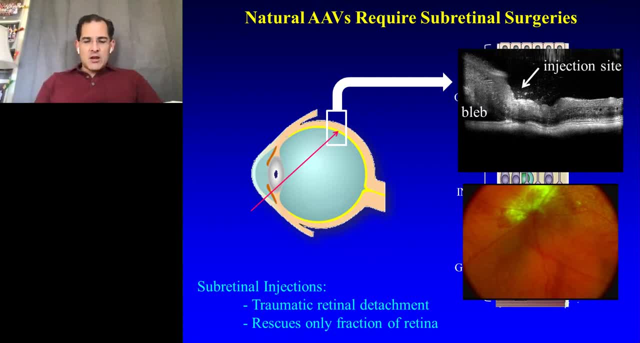 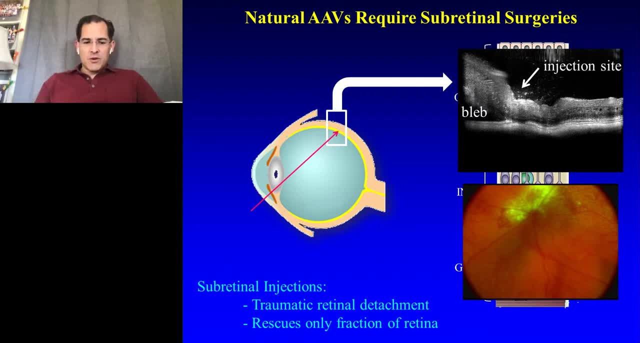 spread only in a small bubble or bleb where the fluid ends up causing that retinal detachment. So this mediates delivery of AAV to those target cells and only around 5% to 10% of the surface area of the retina. So in that FDA-approved product they're actually sacrificing around. 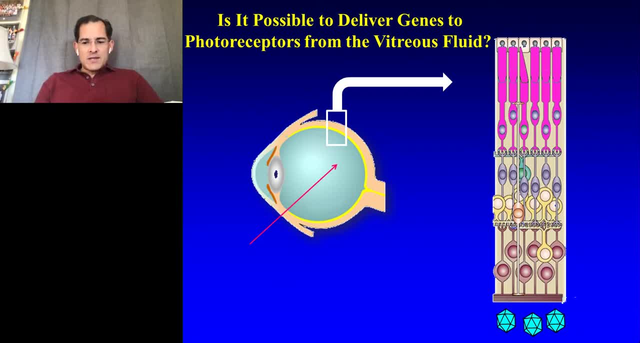 90% of the cells for the progression of the disease. So we ask the question: can we do this? Can we actually evolve AAVs to be able to reach this target cell deep inside a tissue- which is representative of many problems in gene therapy, where you would like the virus to spread throughout? 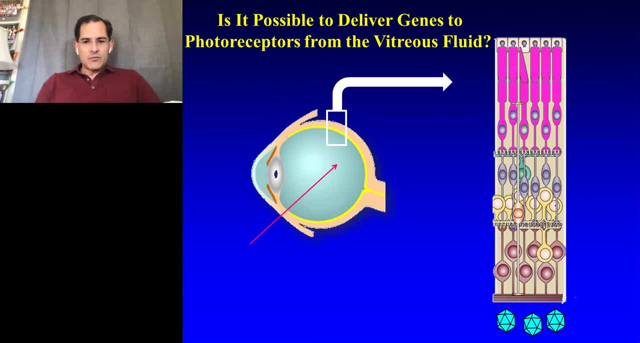 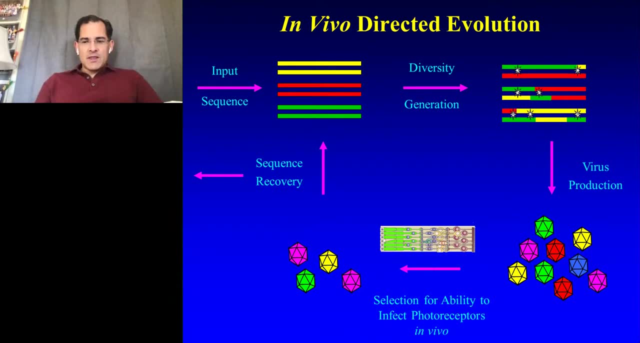 a tissue to be able to reach inaccessible cells. So the way that we did this is that there was no cell culture model that was capable of recapitulating the complex structure of the retina for a long enough period of time for us to conduct the evolution, So we did this in vivo. 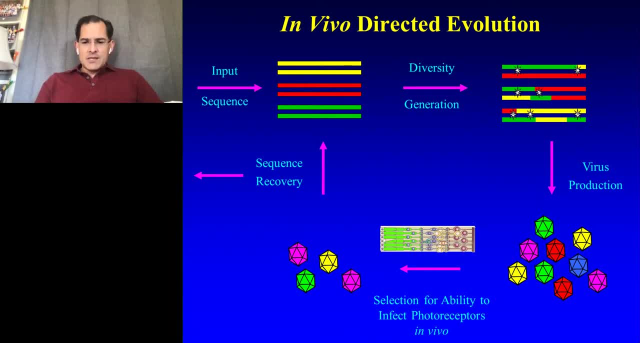 We took our library of viral particles And, in sum total, at that stage our library size was around 100 million different AAV variants. We then administered these, initially in a proof-of-concept study, into a mouse retina, waited a certain amount of time for the winners to be able to traffic back to the photoreceptors. 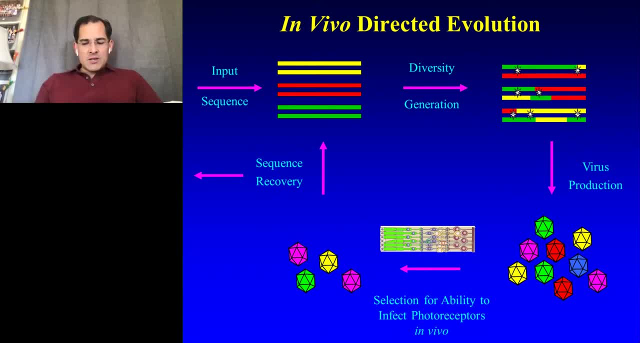 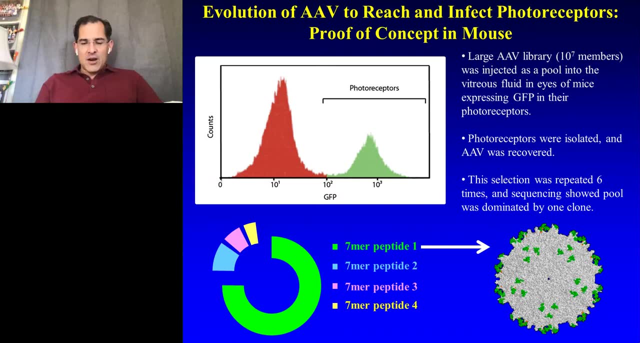 shown in the bottom in green. We then, using fluorescence-activated cell sorting, recovered the AAV genomes that made it to those cells, because those particles carried the DNA then encoded the viral particle along for the ride. You could think of them as being 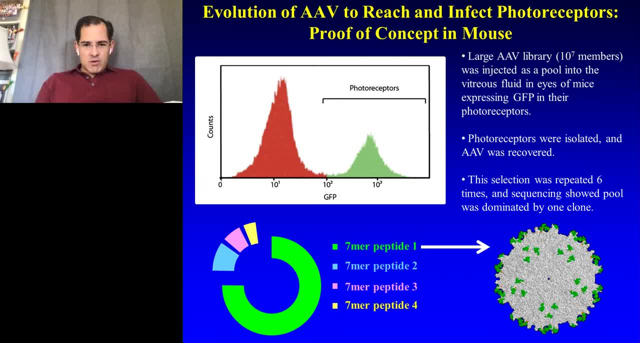 bar-coded with their own DNA. And then we repackaged, the library, readministered it, went through six rounds of selection so that that initially very rich pool ended up converging just down to a small handful of AAV variants shown there on the bottom left-hand. 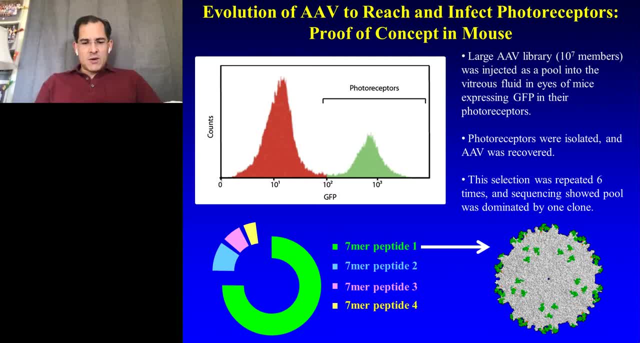 corner with one particularly dominant variant which comprised around three-quarters of the pool. That particular variant, which we called 7-M8, has a structural cartoon shown on the bottom right-hand side, where we see in green there were very single cells And then there were three-quarters. of those single cells, And then in blue there were three-quarters of those cells, And then in red there were three-quarters of those cells, And then in blue there were three-quarters of those cells. So what we did, which we call the 2M1 variant, which we called the other three-quarter programs, 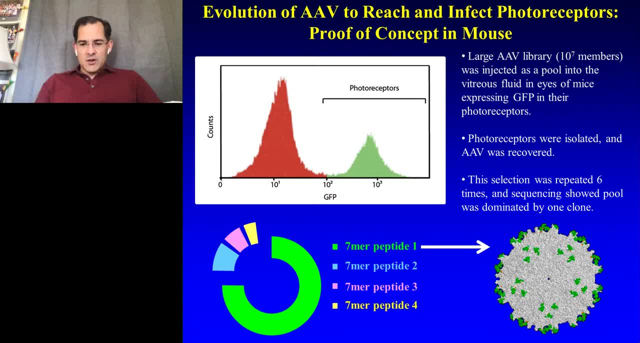 green. there were some changes in the amino acid composition on the viral surface. Specifically, a peptide was inserted into that region of a very specific sequence And you can also see some dots in red. So we had some point mutations as well within that variant. We wanted to test the ability. 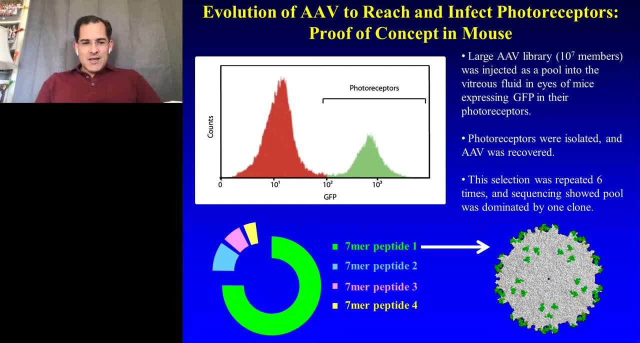 of that variant to start carrying recombinant DNA inside of cells. So we initially loaded it with DNA encoding the green fluorescent protein and began to test its delivery properties in the mouse eye compared to a parent virus, specifically AAV serotype 2.. So shown there, on the bottom left is 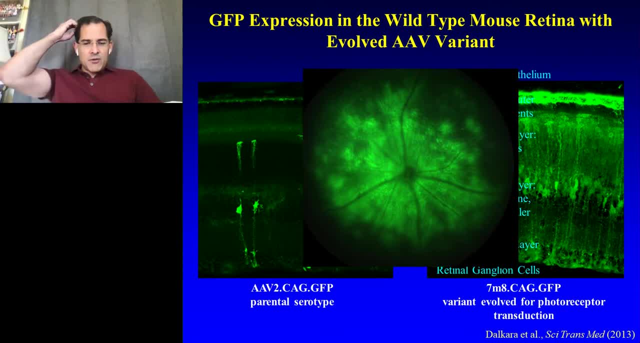 AAV 2. The vitreous fluid is on the bottom side, The photoreceptors are on the top. See why in that FDA approved product they have to use a needle and a subretinal injection to place the AAV right. 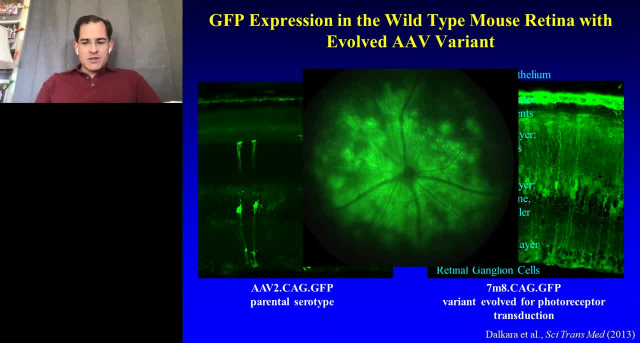 next to the photoreceptors, because AAV 2 from the vitreous can't even reach the photoreceptors. So this compares to the variant that we created- 7M8, where you can see that the AAV 2 is on the bottom left. So this is a variant that we created- 7M8, where you can see: 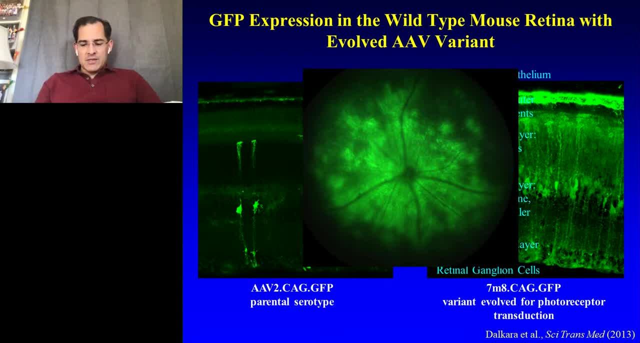 that the AAV 2 is on the bottom left. So this compares to the variant that we created- 7M8, where you can see it. So we're carrying GFP. we're comparing the DNA to every single roughly cell population. 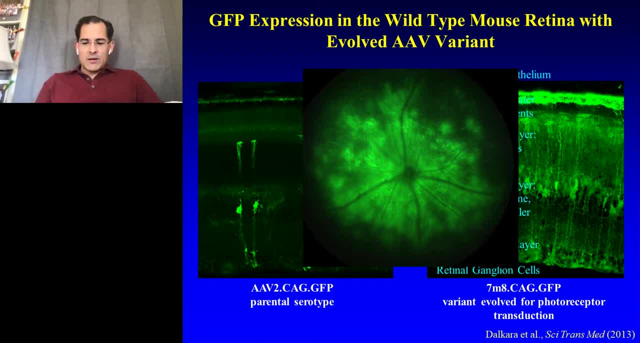 all the way from the bottom, the retinal ganglion cells, to the top, the retinal pigment epithelium. And, furthermore, we're doing this across much larger surface area than 5% to 10% of the retina. we're actually delivering DNA to the full surface area of the retina. So this was an initial proof. 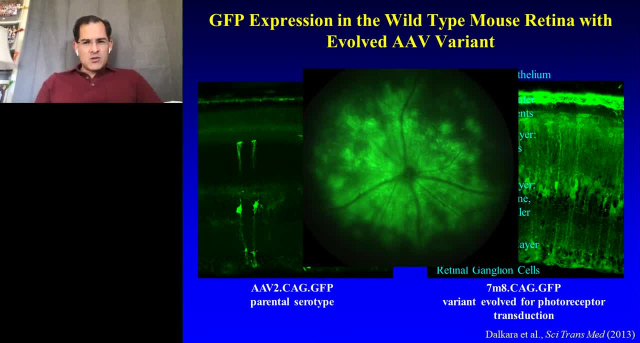 of concept study within mouse And we wanted to test how well it translated to larger animals- And we didn't necessarily anticipate it would translate well to, for example, to a primate. simply because evolution teaches you: you get what you select for. we selected and erode it. we got a. 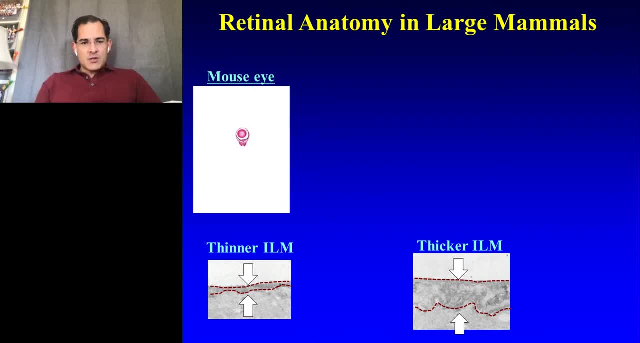 really good rodent factor and the structure of the rodent eye is quite simply different from that of larger mammals in a couple of ways. shown here is size, that as you move from a mouse to a dog, to a, a monkey, a cinnamolgus macaque, to a human eye, there's an increase in the size of the retina. 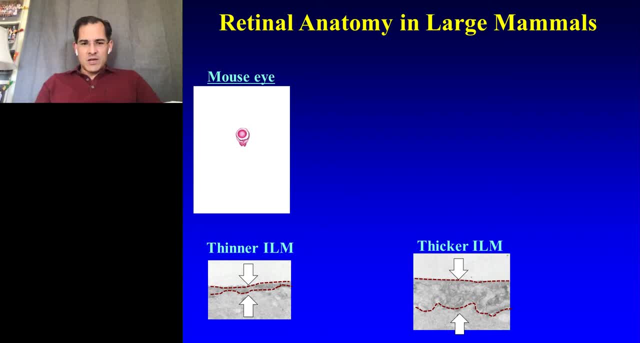 where a mouse has on the order of a hundred microliters of vitreous fluid, whereas a human has four thousand microliters of vitreous fluid and macaque is closer to three thousand, and there's some structural differences as well. um, just wanted to remind you that this phobia is 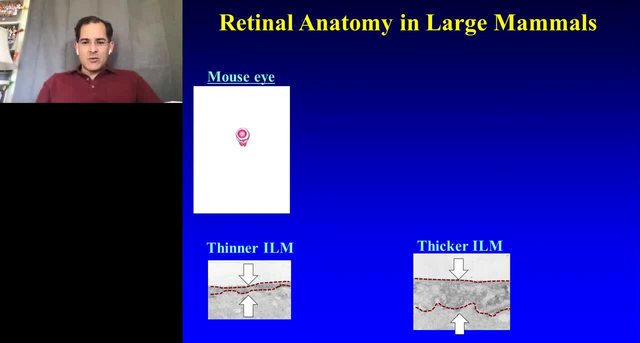 the region of the back of the human eye that is responsible for high acuity vision. it's a particularly important region to protect. mice don't even have a phobia, so you can't uh study the effects of gene therapy on protecting the phobia very well within a mouse. in addition, 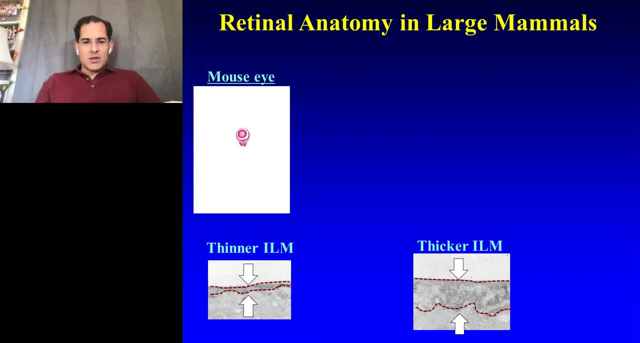 there's a, a, a matrix barrier, extracellular matrix barrier, that lies between the fluid of the eye and the, the retina, the neural retina, and that's called the interlimiting membrane, and it's been shown in a number of studies by ourselves and others that this poses a 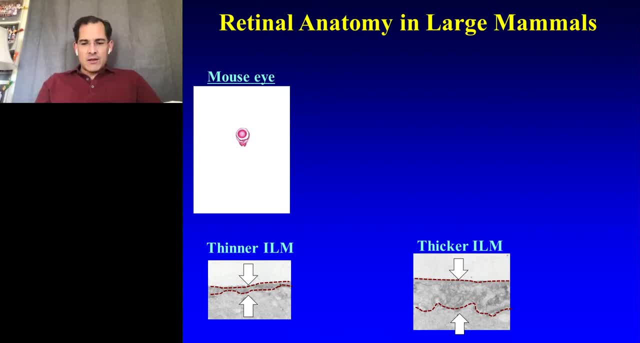 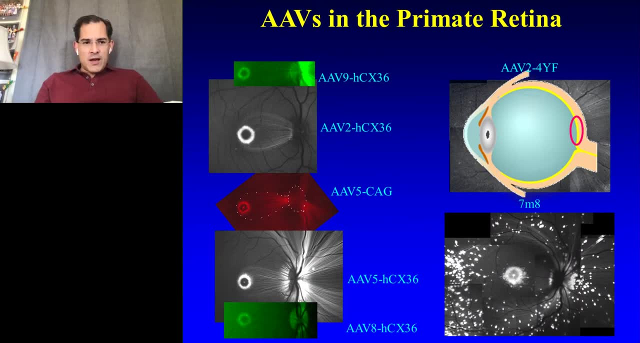 significant barrier to gene delivery and that ilm, that layer is quite simply thicker within larger eyes such as- uh, monkey and human. so we wanted to test what, how this mouse variant did within within macaques, within animals, monkeys rather- and so we tested using a number of natural versions of av av9, 2, 5 and 8, and what we see is this: this transduction pattern. 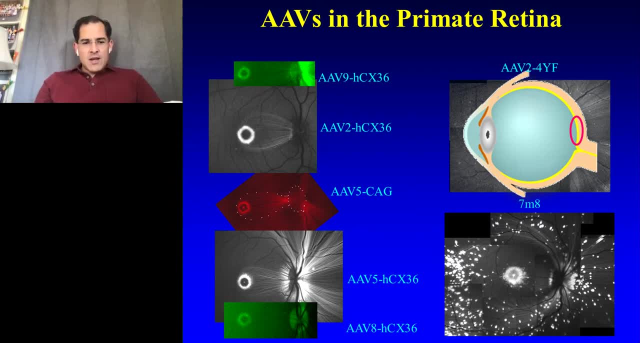 on the lower right hand side you can see the region. the reason for it that the interlimiting membrane is pretty thick across the majority of the surface area of the retina. it thins out right around the phobia and in that region it begins to expose some of those superficial neurons, those 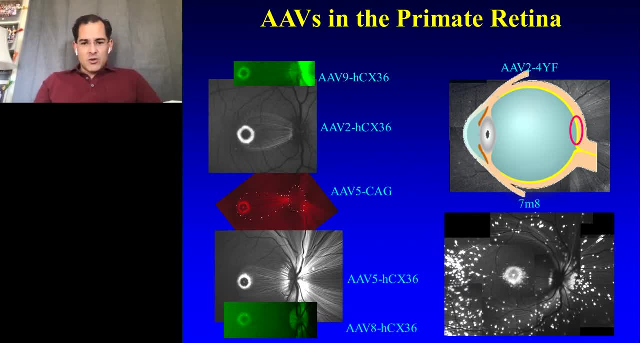 retinal ganglion cells that kind of encircle or surround the phobia region, and so you end up with a ring of transduction around the phobia, a ring of retinal ganglion cells. but on the bottom of the bottom right hand side you can see those cones, those important cells you'd like to protect. 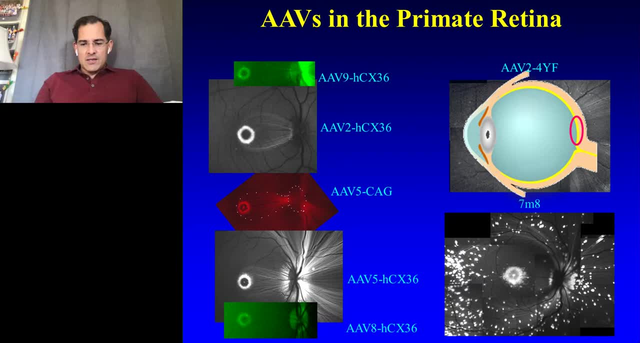 and if this variant were, if these variants were delivering dna to those cells, you would see white in the interior of that circle. but you can see there is none because those natural versions of av aren't reaching those cells. so this is the variant 7m8 that we created. we can see there's better transduction across a number of. 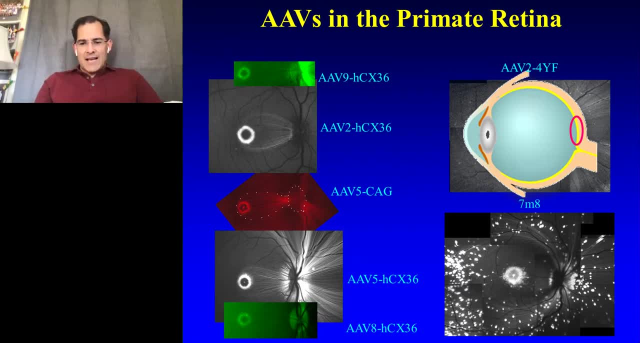 regions across the retina and those turned out to be regions where the vasculature within the retina actually resulted in the thinning of that inner limiting membrane and, in addition, we can see in the middle of the eye that phobia. we do have some transduction, some delivery to cone. 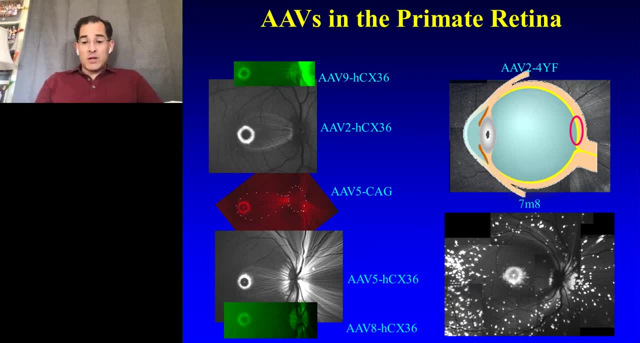 photoreceptors. so it's better than the natural versions, but we felt we could do even better. we're not getting broad, widespread, uniform transduction across the retina, so however this, this variant was, was deep enough to be able to treat a particular condition that was not a normal. 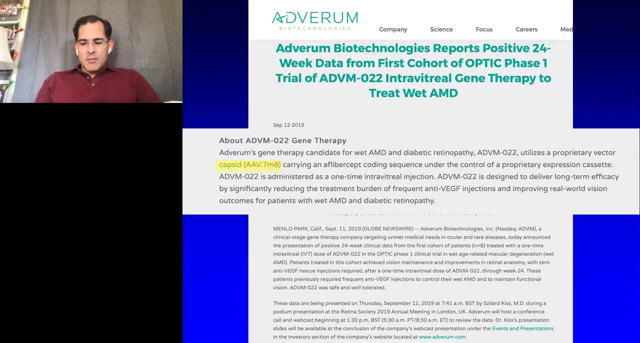 condition um, age-related macular degeneration, and a company down in menlo park known as an aviram i. just i wanted to mention that i had no affiliation with this company, but they licensed uh, this variant 7m8 from uc berkeley and took it into a human clinical trial back in november 2018. 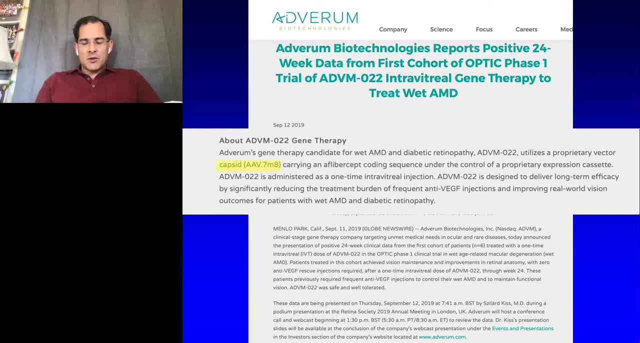 to carry a dna encoding an anti-vascular endothelial growth factor inhibitor to be able to treat patients with wet age-related macular degeneration. and they've reported more recently- as recently as january now- that the first cohort of six patients who were dosed back 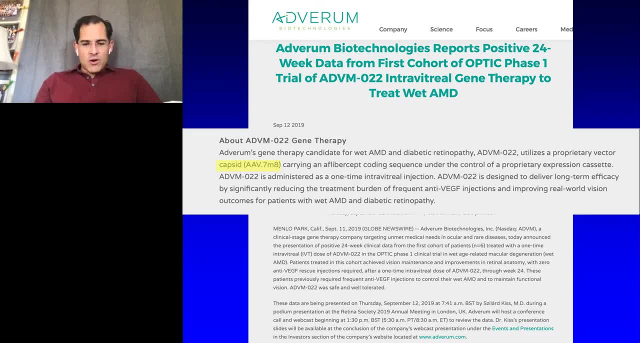 starting in november of 2018, have now, for a period of approaching a year and a half, been off the protein therapy that i mentioned to you earlier. there are anti-veg protein therapies that are injected into the eye on the order of 10 times a year, drugs that were manufactured or produced by 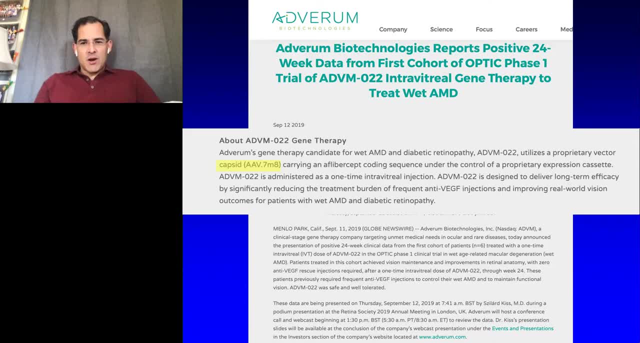 by genentech and regeneron. so these patients have been off of those monthly injections of the protein therapy for almost a year and a half now and they, their vision, is stable and the structure of the retina appears to be stabilized as well. and this is just showing that that press release specifically calls out that variant 7ma. 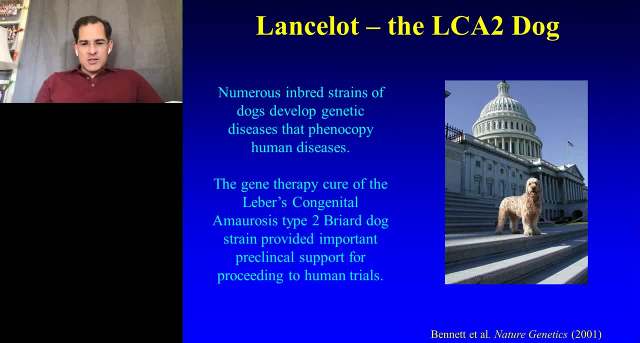 however, we felt that we could do better for the, the gene expression pattern. we could get more widespread transduction across this area of the retina. so we began to move towards larger models of uh of the retina, ones that bore significantly higher resemblance to the human eye, and to do so we started with the dog. so i mentioned to you that fda approved product. 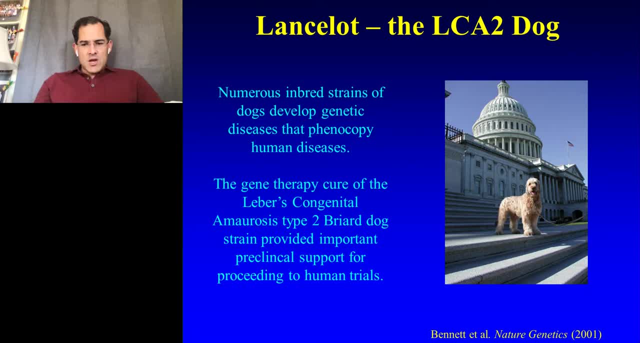 for a blinding condition, libra's congenital amaurosis type 2. in this earlier i mentioned that that particular gene therapy- and it turns out that dog- played a major role in the clinical development or the pre-clinical development of this therapy, specifically because there is a 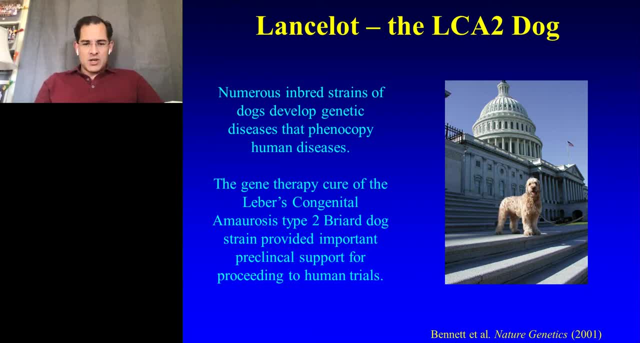 natural strain of dog which has a mutation in that same gene called rp rp65, whose mutation causes that disease within human beings. so we're going to be talking about that in a bit and then we're going to move on to the next slide. so, as a pre-clinical step, an investigator at the university of 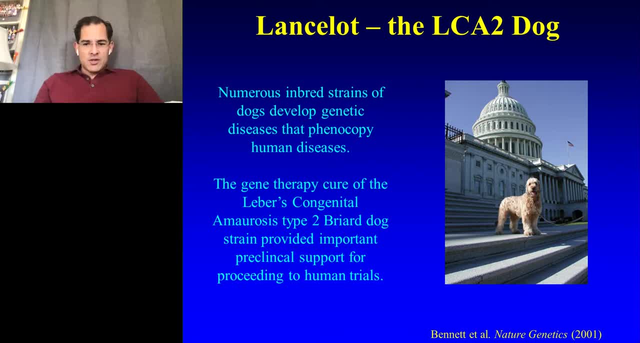 pennsylvania, jean bennett treated these dogs and showed that she could get correction of vision within these animals prior to moving on to human beings and showing therapeutic efficacy within humans. so, in collaboration with william beltran, also at the university of pennsylvania, we began. 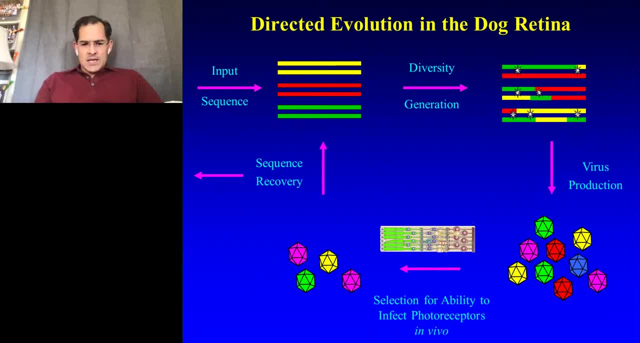 to conduct directed evolution within the dog retina and we repeated the directed evolution, except within dog, and after a number of rounds we were able to detect the metastatic evolution within the dog retina, and so we repeated the directed evolution, except within dog and uh, after a number 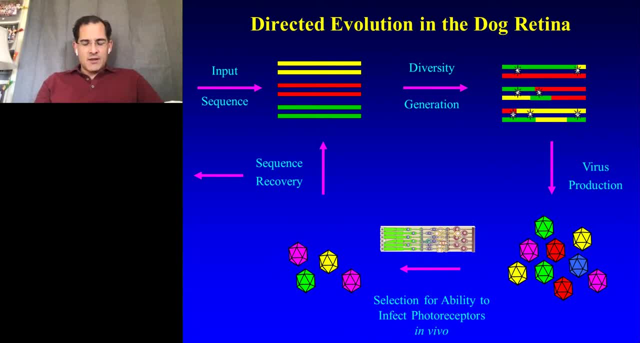 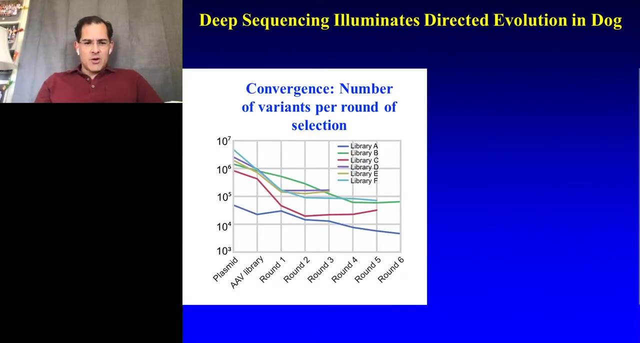 of evolution, we began to isolate some variants of AAV. So one difference between our initially doing this within mouse and more recently within dog is that sequencing technology has gotten a lot better And specifically, we're began to use a luminous sequencing to characterize convergence of our library over time. 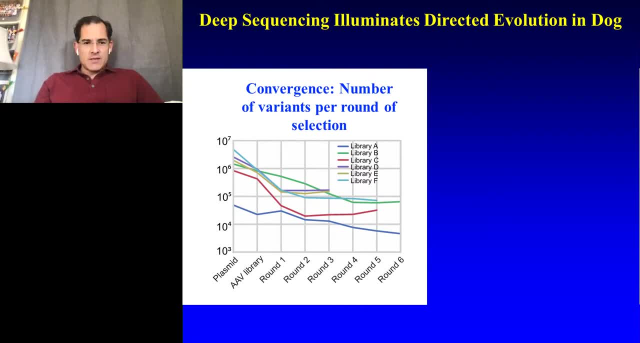 And you can see here A through F. these are a number of different libraries within our pool And specifically, these are libraries in which we made changes to a specific small stretch of the surface of the capsid, for example by inserting a random peptide sequence into those regions. 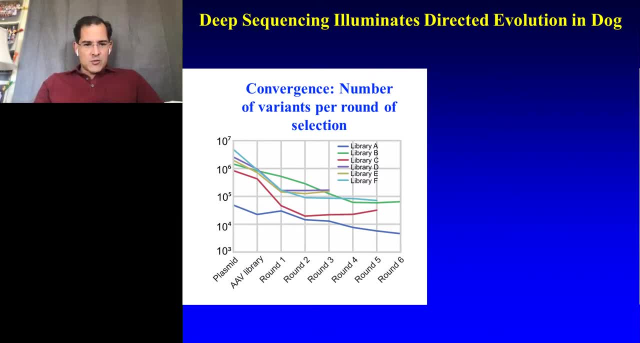 And on the y-axis you can see the number of independent variants, which ranges typically from a million to 10 million variants for each one of those libraries. And you can see on the x-axis, progressive steps in the evolution process, where the first line is plasmid. 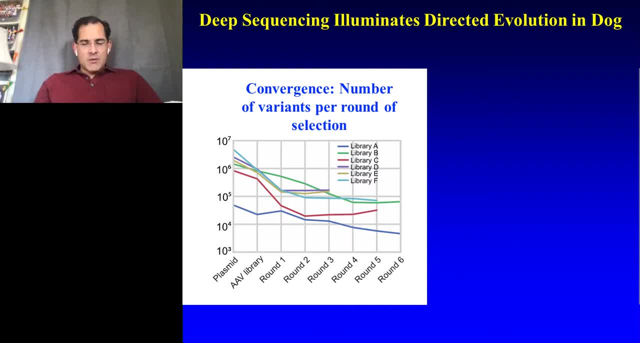 that's the original library as we cloned it. AV library means we've packaged it once, and packaging into recombinant virus plays or exerts a selective pressure where not all of the changes that we made into the capsid are going to result in capsids that can stably fold. 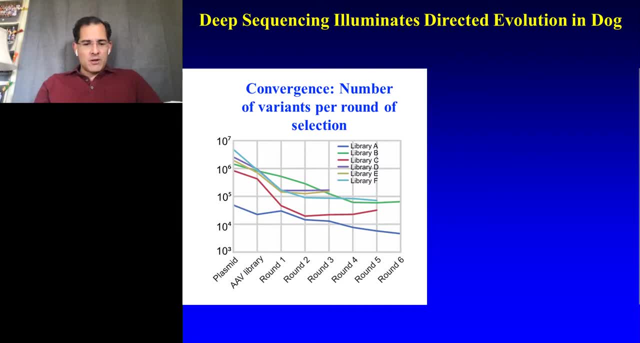 So we see a selection there for packageability, if you will. And then rounds one through six were progressive rounds of selection for the ability of those variants to reach target cells inside the eye. We observed something interesting in the original library. to begin with, this is the plasmid. 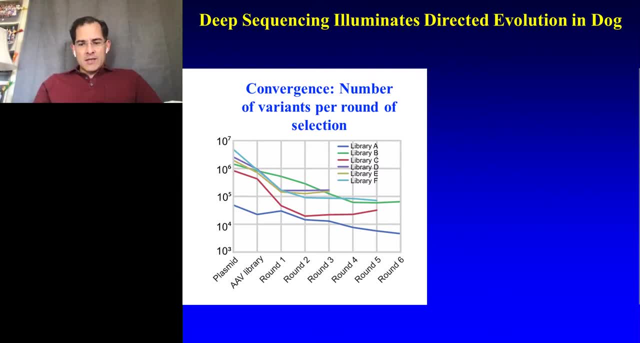 library And ordinarily, you would ideally like to see that every single recombinant variant had an equal shot on goal, had an equal opportunity to be able to show off, to be able to reach the retina, But some of these have actually stacked the deck. 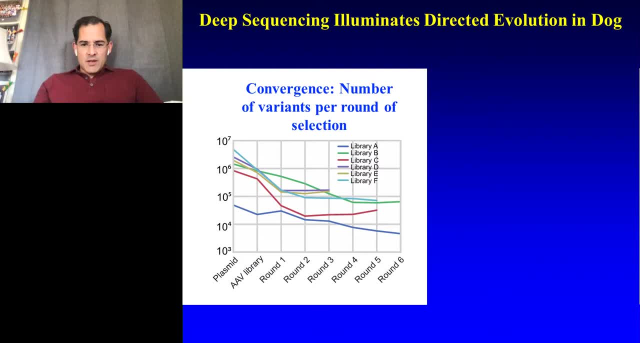 And on the left-hand side, you can see that there are some where there's a significantly higher abundance relative to the majority of variants which are equally represented, as indicated by the fact that most of those curves have a flat line towards the right hand side. 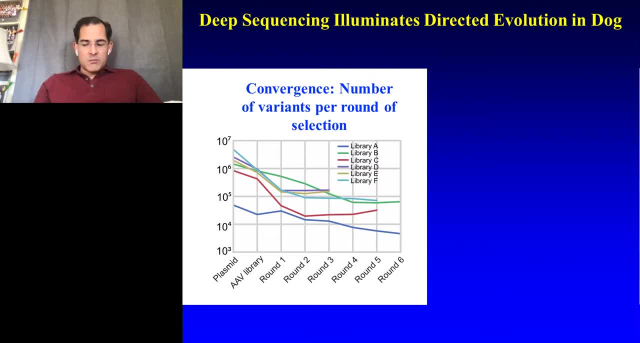 But on the left-hand side you can see some variants. due to, we believe, artifact associated with a ligatively tied DNA synthesis from DNA synthesis companies where we ordered random sequences from those companies, There was some bias that led some variants to be represented as much as 100 or 1,000 times higher. 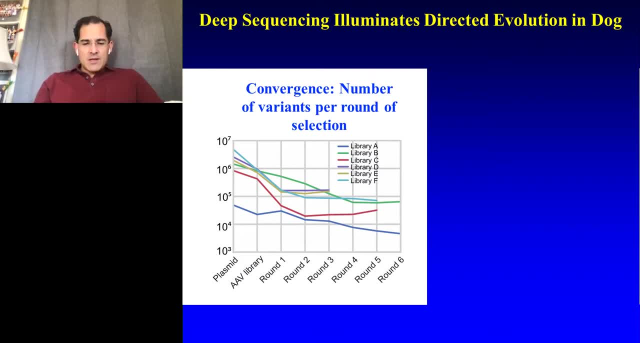 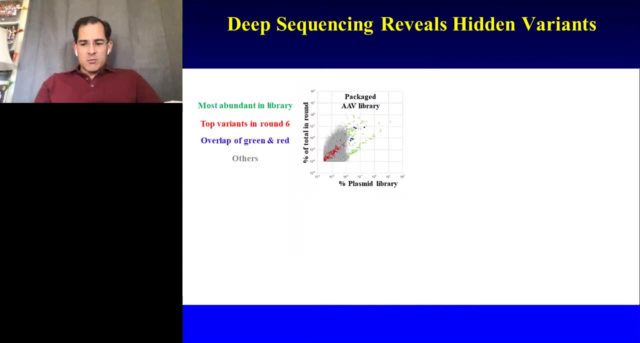 in frequency relative to the rest of the members in the library. So to be able to make sure those variants didn't have an unfair advantage, we conducted evolution in which we sequenced the distribution of variants, which actually we called an evolution of variants emerging. 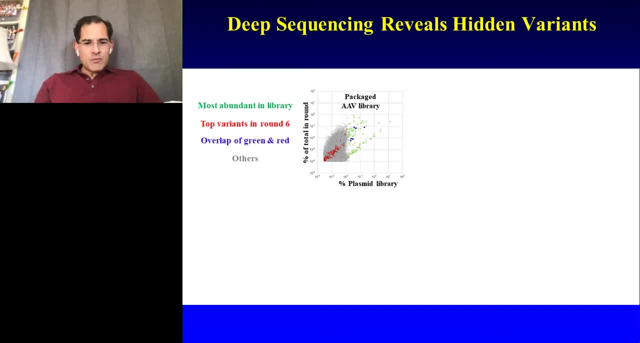 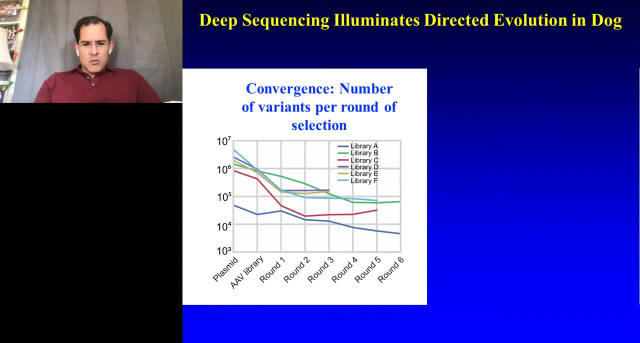 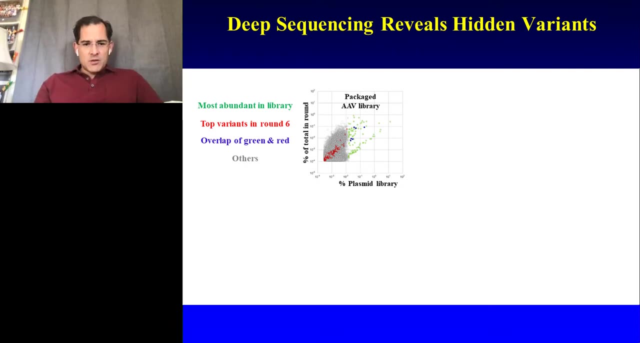 from the Darwinian selection every single round along the way. And this is the selection, And I'm going to run through this. Sorry, We're on the y-axis. We have the percentage of each one of those variants. Each variant within the pool is represented. 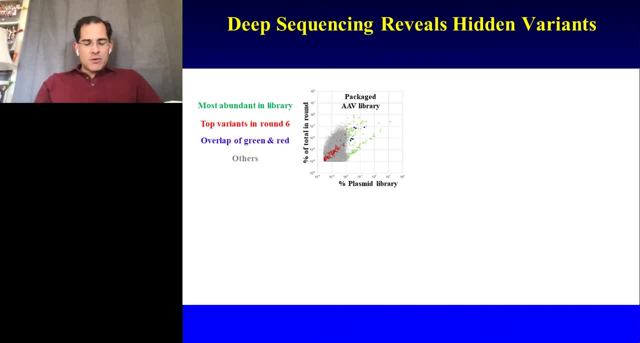 as a single dot in that dot plot where the y-axis shows what percentage of the pool comprised after it was packaged. in that first plot after round one, two, three, four, five, six axis that is compared to the percentage of the frequency. 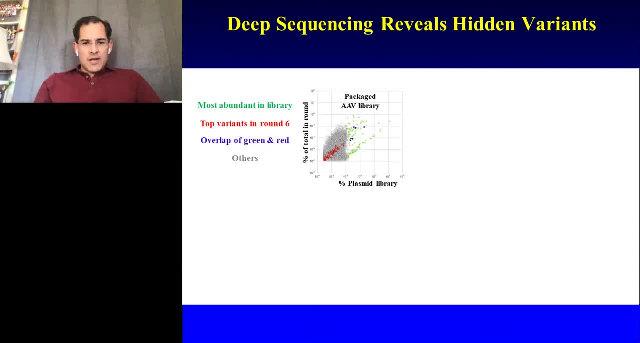 of that variant within the original plasmid library. So what you'd like to see is that some variants should of course stay in the same position on the x-axis because they had a particular presence, a particular percentage or frequency within the original library. 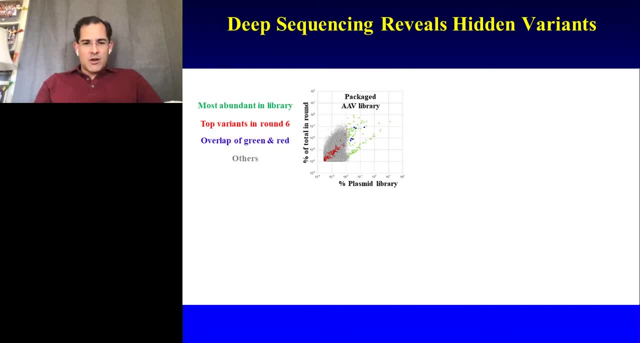 but you'd like to see some rise up progressively higher and higher on the y-axis, indicating that they're being selected, for they're increasing in frequency as a result of the evolution process. Furthermore, the ones that had an unfair advantage to begin with are shown there in green. 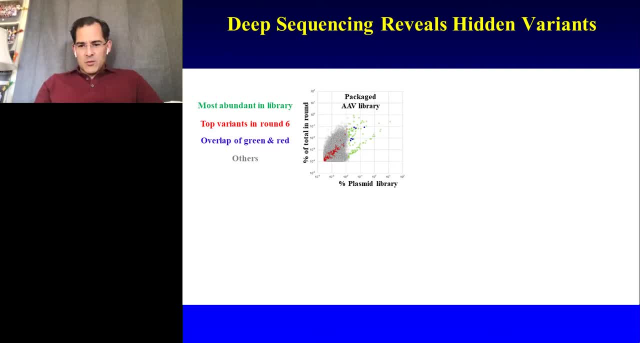 and the ones that ultimately are the winners after round six. you can see in the lower right-hand side shown in red. those are the most frequent variants within round six. You can see where they lay. within the original rounds There were low frequency variants. 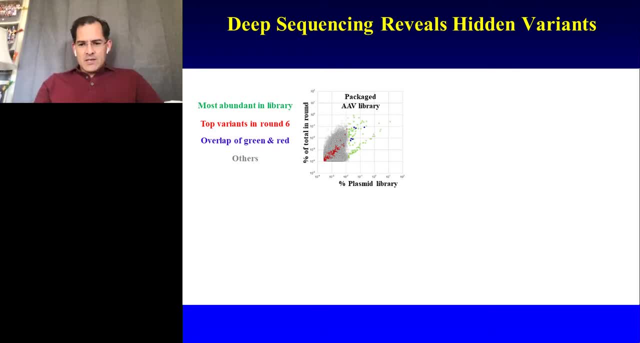 but progressively climbed the y-axis over time, And so the ones we really focused on were the ones that were red but not blue, not the ones that were the most abundant within the original pool, And those were the variants that we wanted to then test. 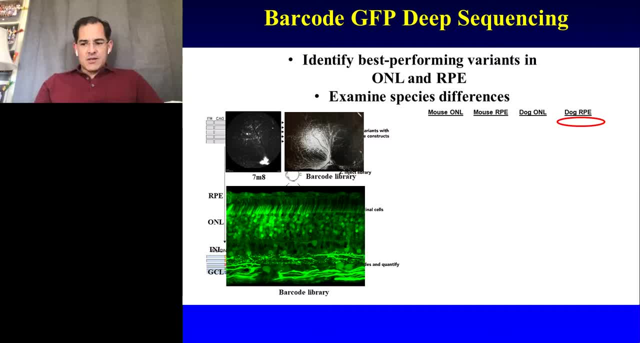 So the way that we tested them is that each animal subject is quite precious, both for ethics as well as economical reasons. So we took a number of different variants- on the order of 20, and we used each one of those capsids. 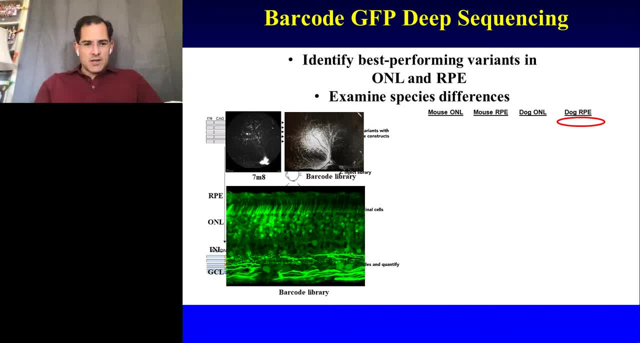 to package a particular genome that contained the green fluorescent protein and also contained inside of it a small barcode, a molecular identifier, where the identity of that barcode shown in the upper left-hand corner there of that plot there was a one-to-one correlation or relationship. 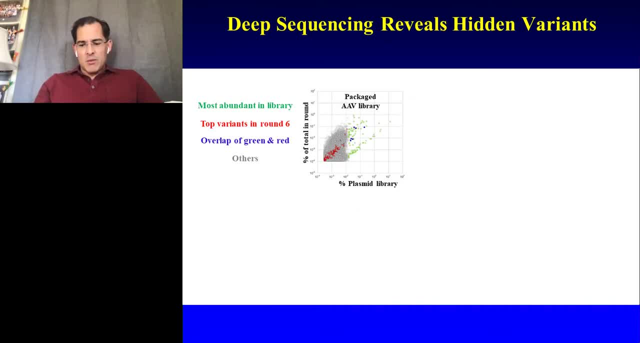 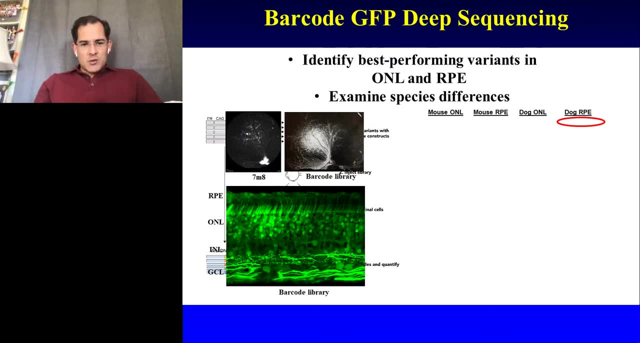 between the sequence of that barcode and which of those variants shown in the bottom right-hand corner in that circle, which one of those red variants was used to pack that barcode. So we packaged 20 different barcodes with 20 different capsids individually. 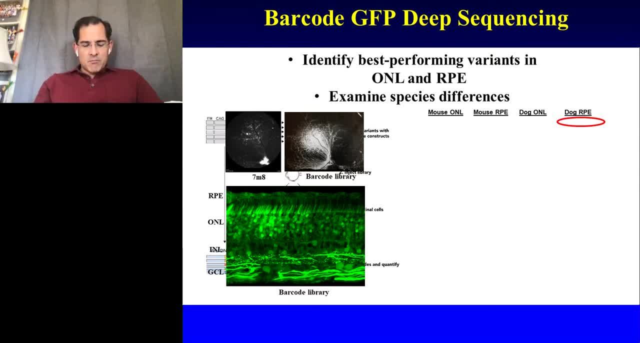 and then pooled all of them together, administered, mixed them together, injected them into the retina of a dog and then both visualized the retina. So you can see here that we have a large number of cells that are expressing the green fluorescent protein. 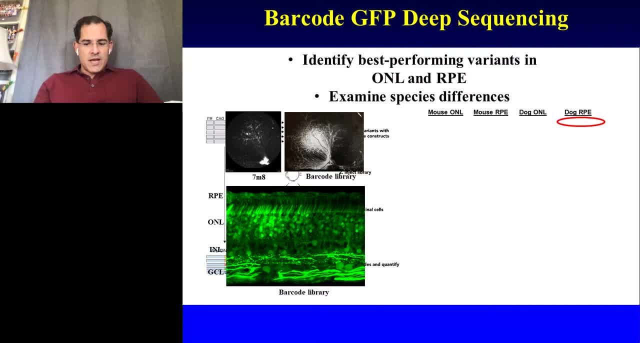 which means that at least one or more of those variants of AAV- the new variants that we created- were capable of carrying their DNA deep inside of the retina. However, we can then isolate the photoreceptor neurons and use DNA sequencing to recover the frequency. 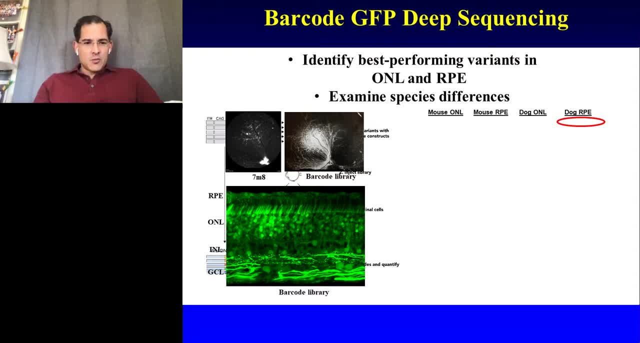 of those barcodes within that tissue And that tells us which capsids were capable of carrying DNA very efficiently inside of that tissue and which variants were capable, as a result, of mediating the expression of high levels of GFP, high levels of messenger RNA, within those cells. 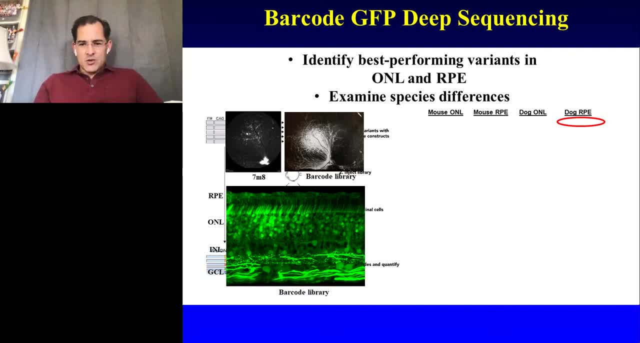 So we took our entire pool, We applied it into the mouse just as a control, and then we applied it within the dog And we can see a number of interesting features here, shown on the right-hand side. You can see that, regardless of whether we apply it, 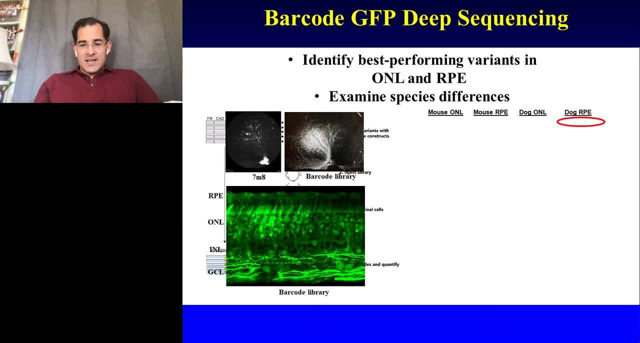 to mouse or dog. AAV2 is near the bottom, indicating that that natural version of AAV is not very effective. On the right-hand two columns we can see that the variants that we call canine canine, number nine and number 16,. 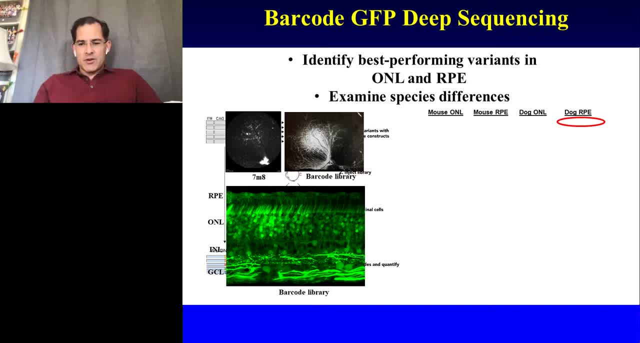 were very effective at being able to mediate delivery and genic expression within the dog. But if you take a look within the mouse, canine nine and 16 are a little bit lower than the dog and this tells us that there's sequence specificity. 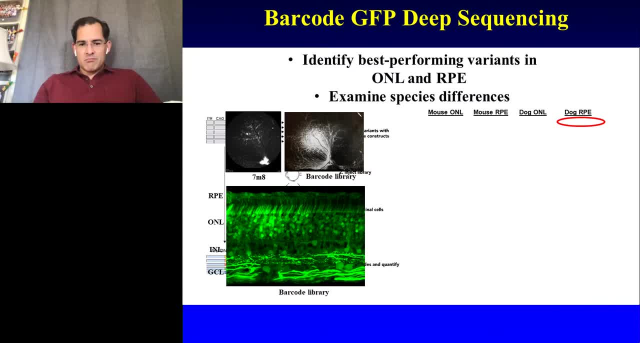 for which a variant is optimal. Again telling you that nature teaches us to get what you select for in an evolution. So if you want to create variants that are optimal within a larger animal model, that tells you you can't do the selection within the mouse. 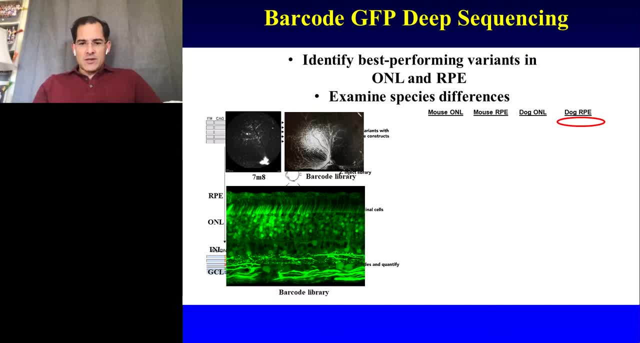 You have to do it within the larger animal And you see the converse as well, that the top variant within the mouse- canine 12, is actually lower on the list within the dog. So we took the top variant, canine 16,, and we then 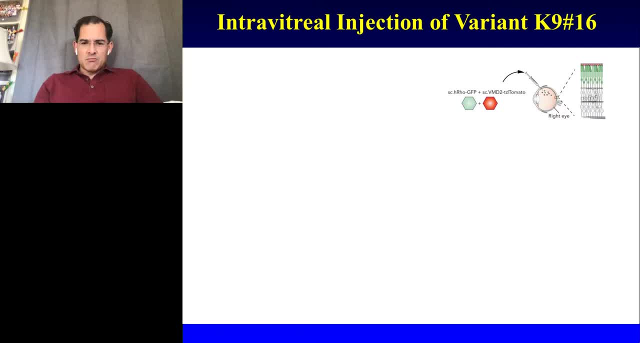 tested it individually within the eye and we actually generated two genomes just to test its ability to mediate delivery both within photoreceptor neurons as well as the other target cell within the eye that I haven't talked about too much yet. 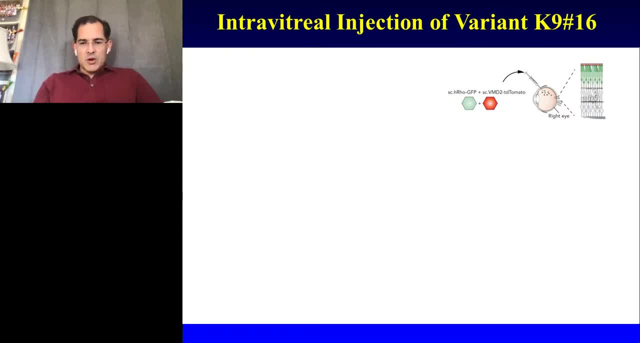 which is the retinal pigment epithelium. So we specifically loaded two different genomes into that variant, one that contains GFP under the control of a photoreceptor promoter and the other one of which contains a TD- tomato or red florescent protein- under the control. 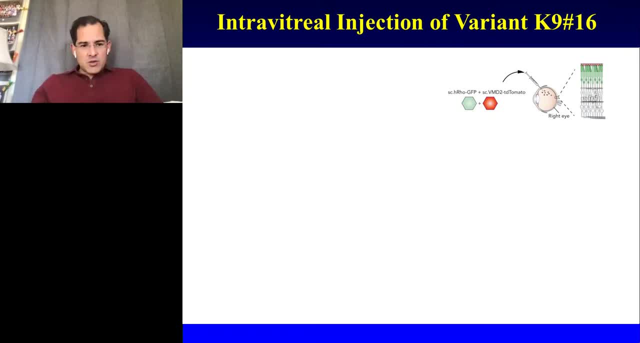 of retinal pigment epithelium promoter. We compared this to the variant within the literature that had been reported to be the best for delivery to the dog eye from the vitreous, a variant called AV24YF plus TV, And you can see our variant here, the canine 16,. 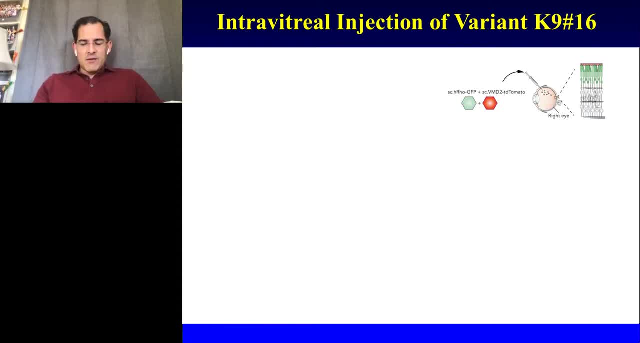 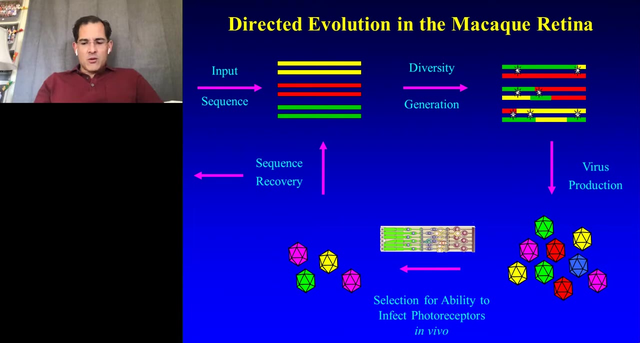 at various levels of magnification is mediating very, very high transduction, very high levels of delivery and gene expression, both within photoreceptor, shown in green, as well as within retinal pigment epithelium, shown in red. So ultimately, we, of course, were very interested. 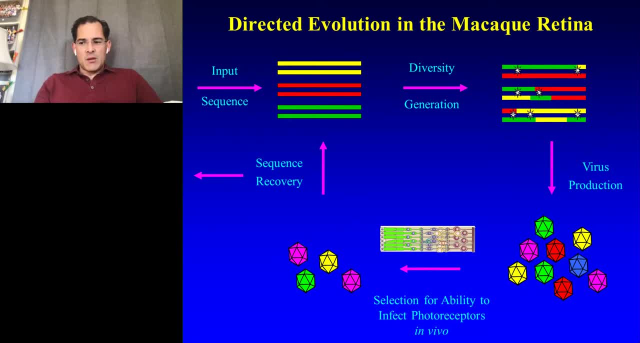 in translating this into the clinic, into human gene therapy, to be able to treat the 200 plus blinding diseases that rob people of their vision. So I'm gonna show you a couple of slides now in which we conducted the evolution within non-human primate, within cinnamulgus macaque. 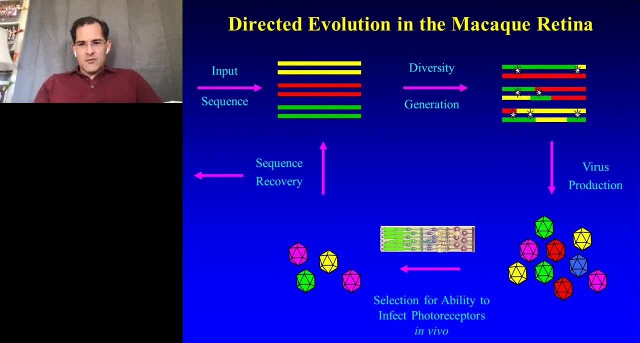 And this was work that was done at a company that I co-founded called 4D Molecular Therapeutics. It's now an 83-person company located in Emeryville, California, And it's a company that is taking these products into human clinical trials. 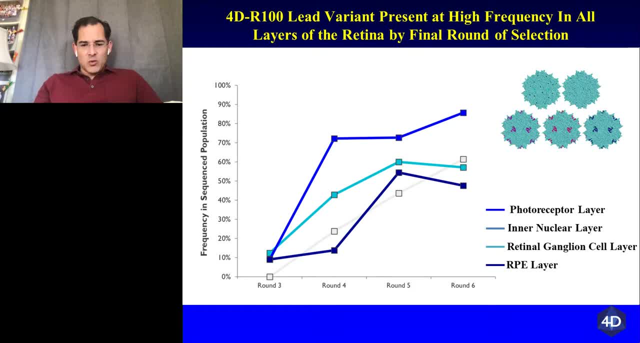 So this is the Y-axis sequencing results, or the percentage of the pool of variants that were recovered after every single round, or at least rounds three through six: The pool that came from photoreceptors, from the internuclear layer and from the retinal ganglion cell layer. 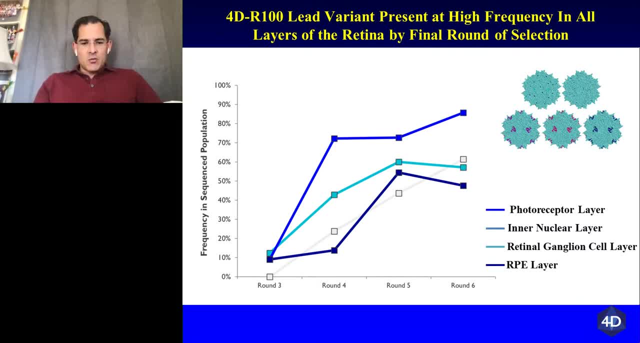 as well as the retinal pigment epithelium layer, And there was one particular variant where you can see that, regardless of which one of these layers you're looking at, it was the dominant variant And that's actually comprising in some cases. 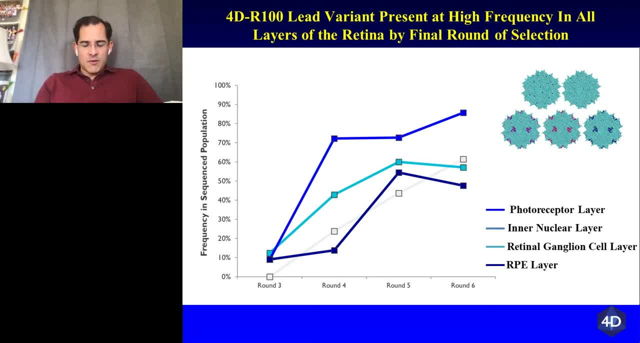 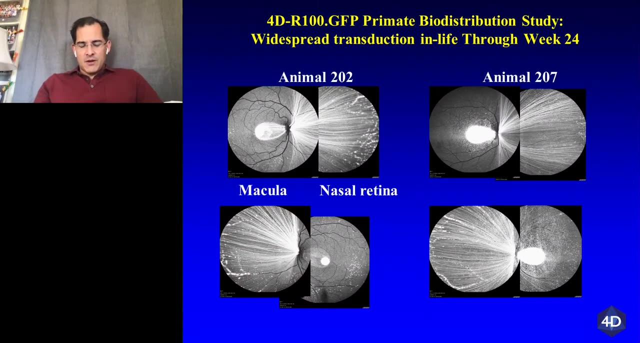 over 80% of the variants that were emerging from that region. We then took this variant, used it to package the green fluorescent protein and began to conduct studies that were IND-enabling, And shown here is a fluorescence live fundus image of. 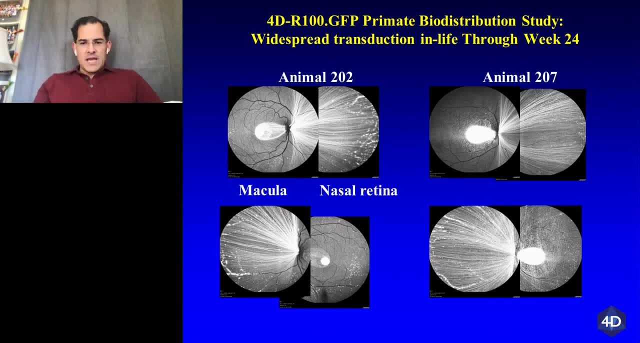 in this case several non-human primates, And you can see that there's a widespread expression at the back of their eyes. This is actually six months after delivery of that AAV carrying the green fluorescent protein into these animal eyes, And we took these animals post-life. 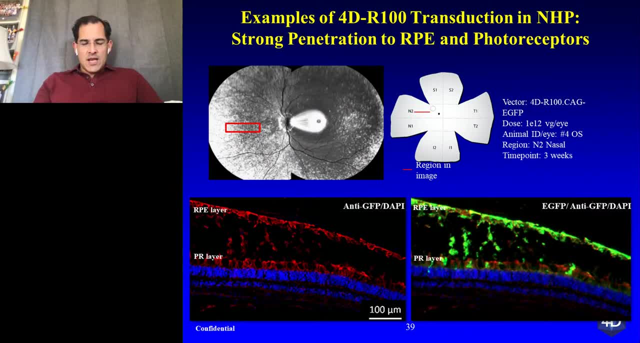 and did literally thousands of histological sections And you can see that some regions are brighter than others. but across the entire retina, even whether it's the regions that are white or gray, in the upper left-hand corner, we see high level of expression of the green fluorescent protein. 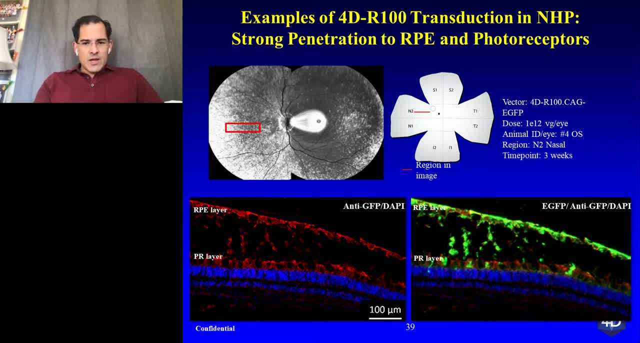 across multiple layers within the retina. So, based on this, we've actually filed two INDs to the FDA. These are now open INDs where we have authorization to initiate human gene therapy clinical trials for X-linked retinitis pigmentosa, as well as for choroideremia. 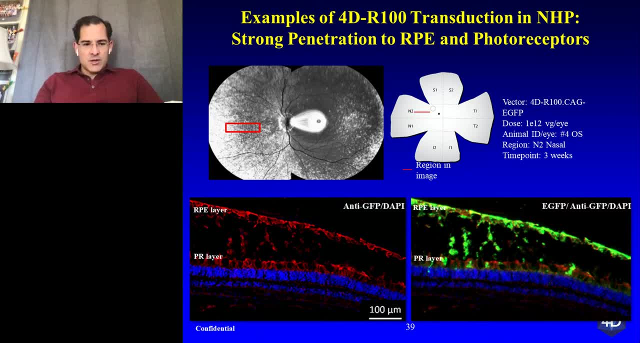 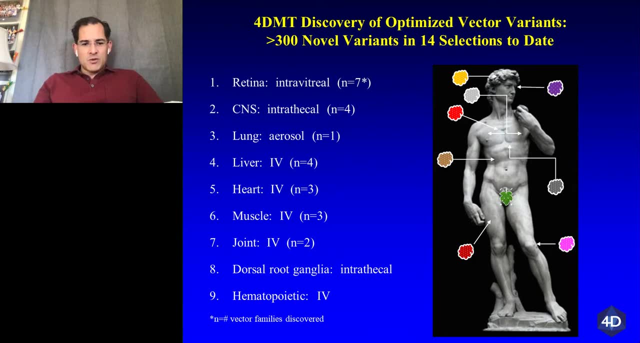 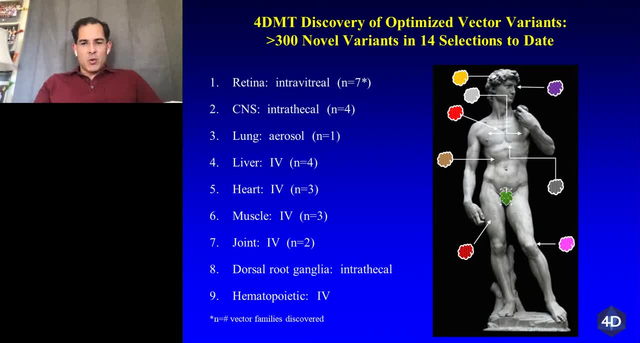 but in the central nervous system, lung, liver, heart, et cetera. so actually 14 selections to date that have resulted in 300 novel variants of AAV that we've created and the next target tissue that we're gonna be clinically pursuing. 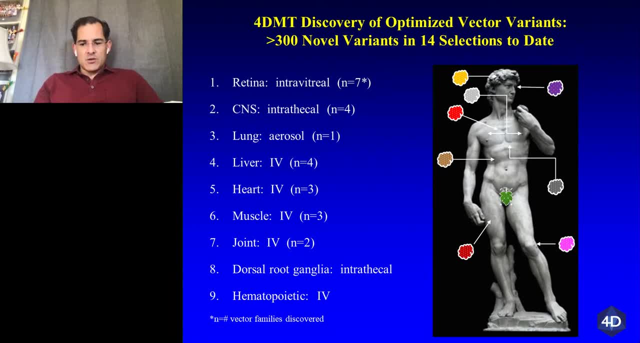 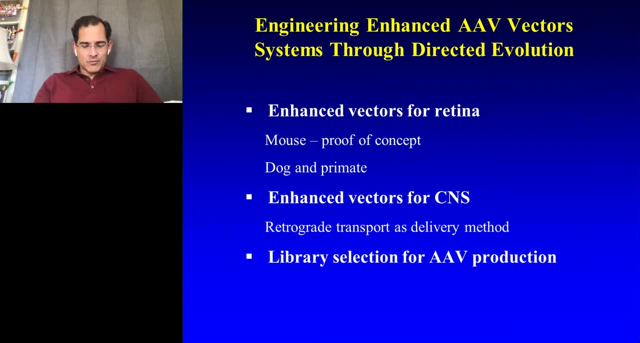 is actually muscle, both skeletal and heart muscle, and we're soon gonna be- this month- filing an IND to be able to initiate clinical trials to treat FabRase. So I'd like to talk about a different mode of delivery for gene delivery in the central nervous system. 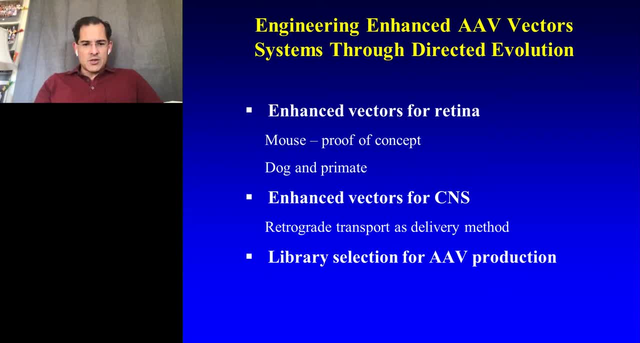 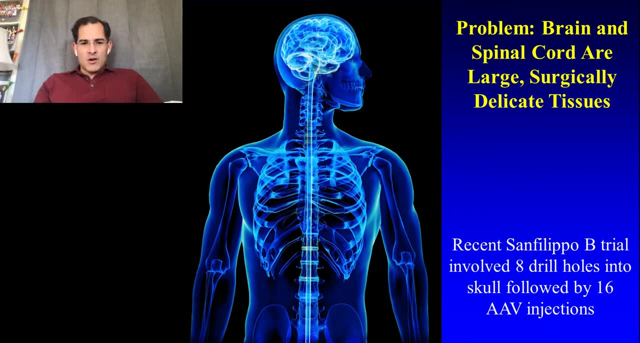 and it's actually a different mechanism of spread of virus into this tissue, a process called retrograde transport. So, whether the tissue is the eye, or the brain or the heart, we have some fundamental problems, which is that these are relatively large tissues. 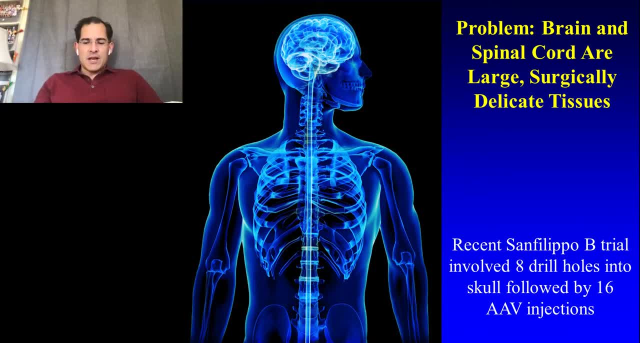 and can be very delicate surgically and it's difficult to get AAV to spread to a large amount of that tissue. So one of the clinical trials that we've done and we've been able to do a lot of research and we've been able to do a lot of research. 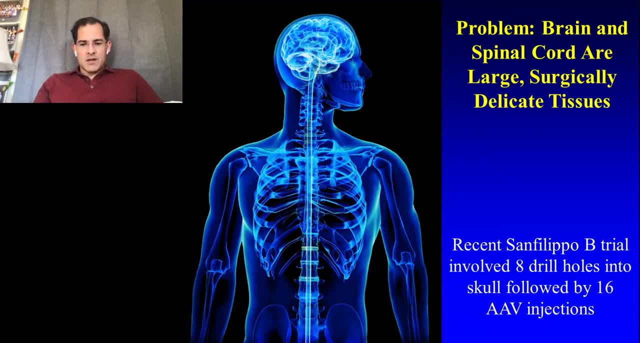 is to look at the cells that illustrated within the brain. this concept or this problem was to treat this lysosomal storage disease called Sanfilippo B and to be able to try to infuse AAV through a majority of the volume of the brain. 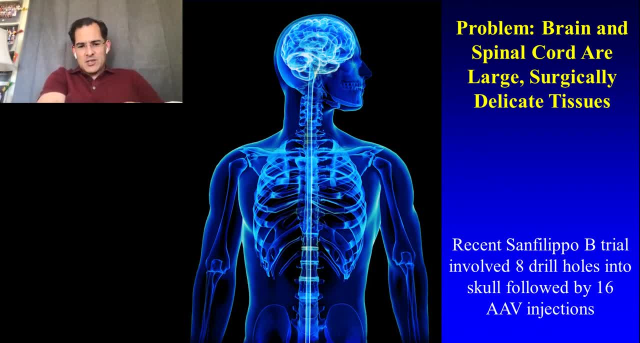 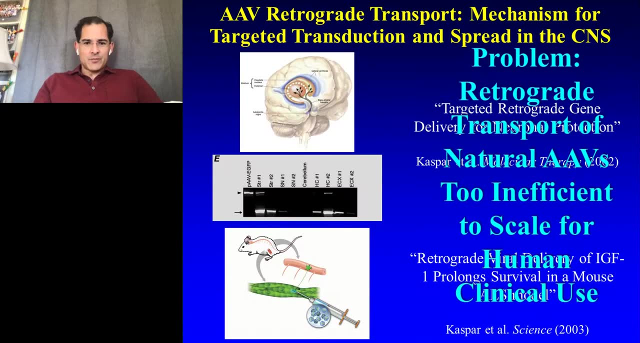 they actually drilled eight holes into the skull and did 16 AAV injections and still didn't restore high enough levels of enzymes to be able to modify the disease. in that condition We co-discovered a mechanism for AAV transport within the brain called retrograde transport. 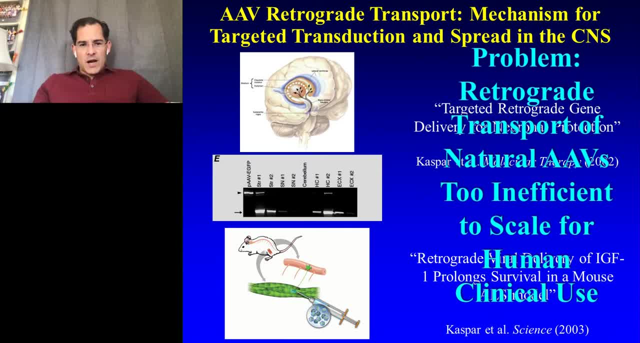 so specifically. we know neurons have a cell body where the nucleus is, and then they extend for the extent of axons, in some cases millimeters or many centimeters inside the body, and we found that if you deposit an AAV right at the end of one of these axons, 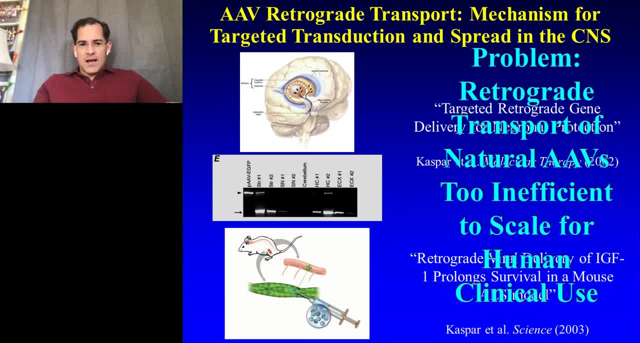 the axon can actually internalize the virus and traffic it back retrogradely along that axon for very long distances- in some cases infect remotely, if you will- And this was utilized subsequently by Brian Kaspar in a study back in 2003,. 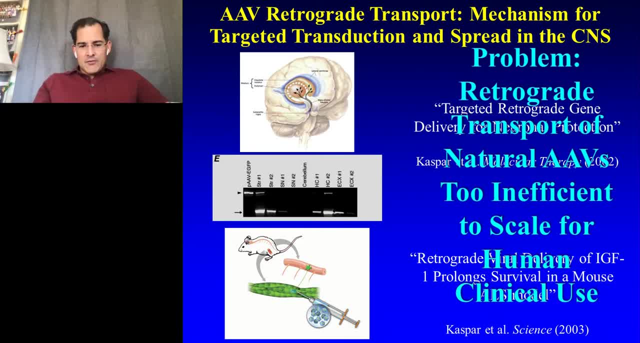 in which he injected AAV into the muscle of a mouse and the virus was internalized by the axons of motor neurons, and the motor neurons then retrogradely trafficked the AAV back to the spinal cord, and this is a way of being able to mediate high efficiency. 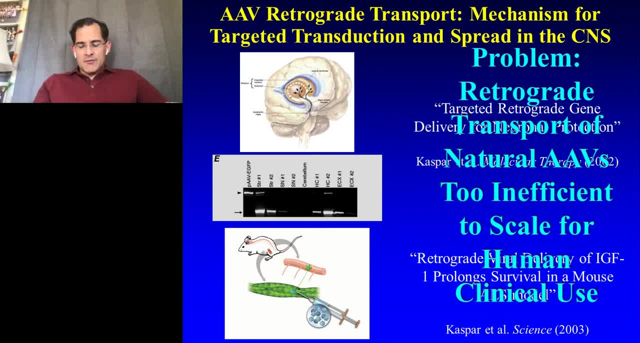 or relatively high efficiency delivery to the spinal cord of that mouse after a simple intramuscular injection taking the virus brain barrier. And he used this to inject AAV into the muscle of a mouse and he used this to mediate a protective factor. 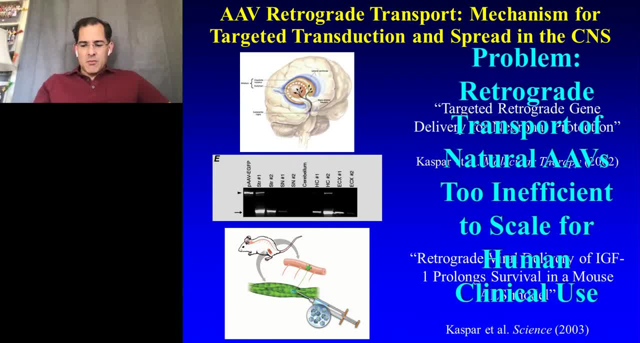 into the central nervous system of a mouse model of amyotrophic lateral sclerosis in this extended animal lifespan. So a company began to develop this retrograde transport technology and unfortunately found out that the efficiency of retrograde transport was too low. It worked reasonably well within a mouse. 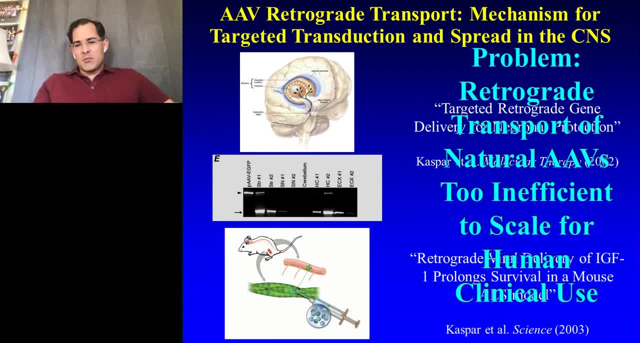 less well within a rat and not well at all within a non-human primate, And so it became to scale up for human clinical use, Even though this could be a very effective approach to be able to get spread within the central nervous system. 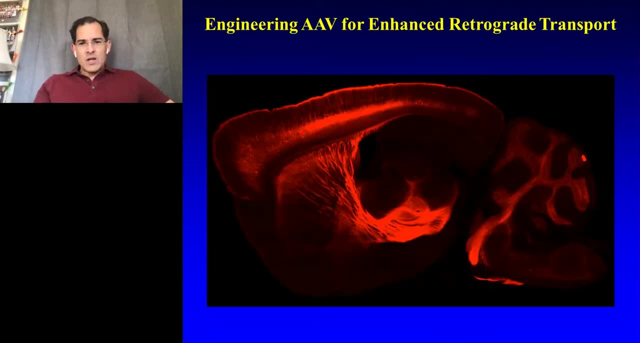 as I'll show you in a couple of examples. So we began to conduct AAV evolution for retrograde transport, and the system that we utilized is shown right here. This was initially done within a mouse, and the cortex of these animals sends projections. 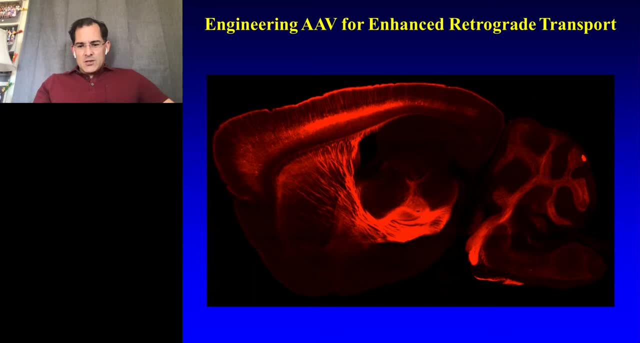 over a long distance to a centralized region called the pons. So the idea is that you could do an injection of the library inside the pons and some cortical neurons would end up internalizing that virus and retrogradely transporting it back to the cortex. 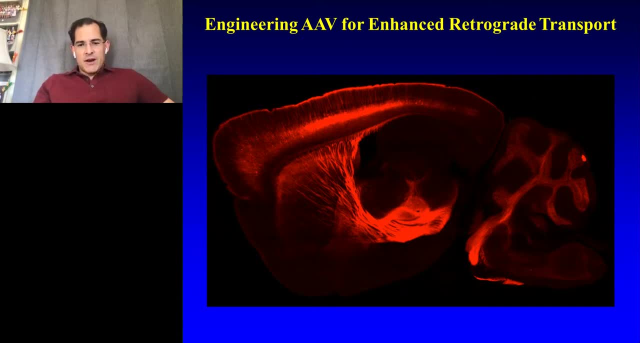 And, as a result, with a single focal injection you could get the virus to spread through a large volume within the cortex of the brain. So we repeated this evolution multiple times and ended up with one dominant variant emerging. We then loaded it with a transgene that would end up. 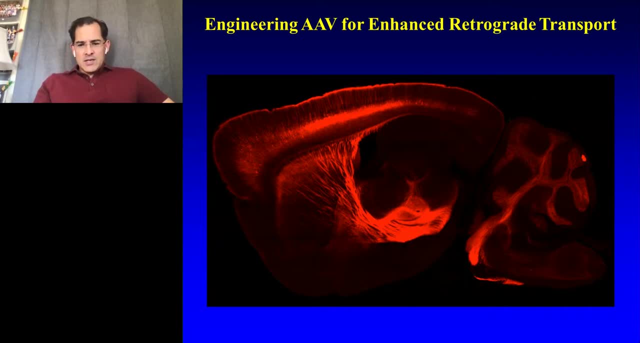 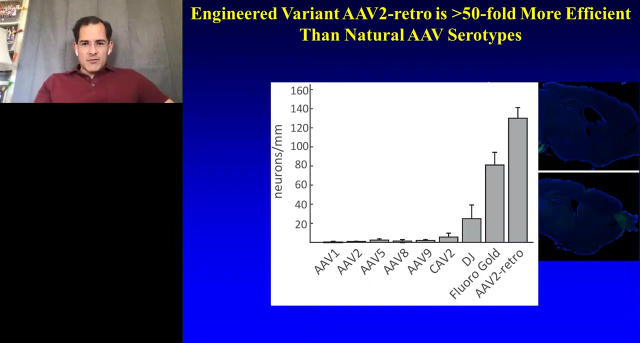 resulting in expression of a TD tomato. And you can see a single injection into the pons resulted in very widespread expression across the brain. So we wanted to quantify the level of increase in this retrograde transport. So we ended up loading several different AAVs with a cargo that resulted in expression of 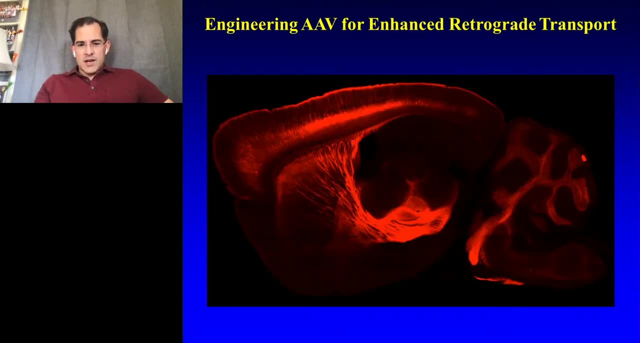 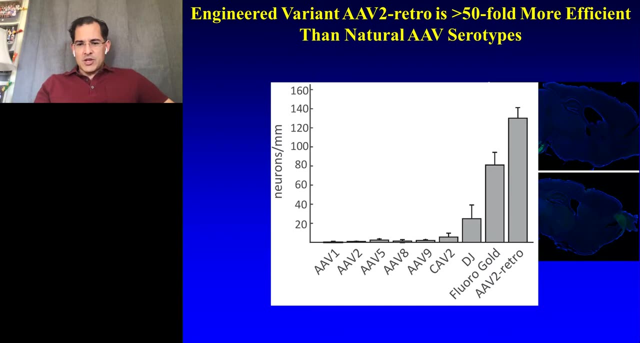 GFP just within the nucleus. This is TD tomato across the cytosol of cells. so it's kind of hard to count individual neurons. This was a nuclearly localized cargo so we can see that upon injection into the pons in the lower left-hand side you should get expression. 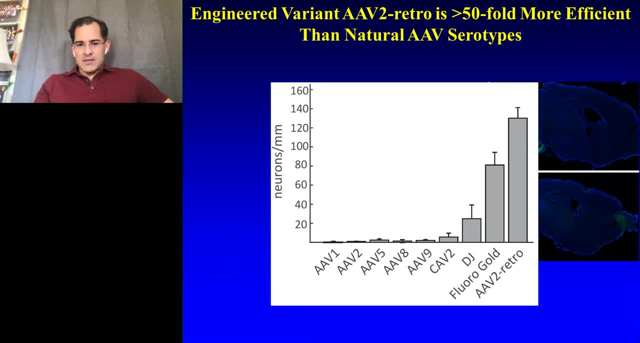 across the cortex In the upper right-hand side. there's none in the case of AAV2.. In the case of this particular variant called DJ, this came out of Stanford. you can see, at least in the bottom panel, that there's some neurons in the upper right-hand side. 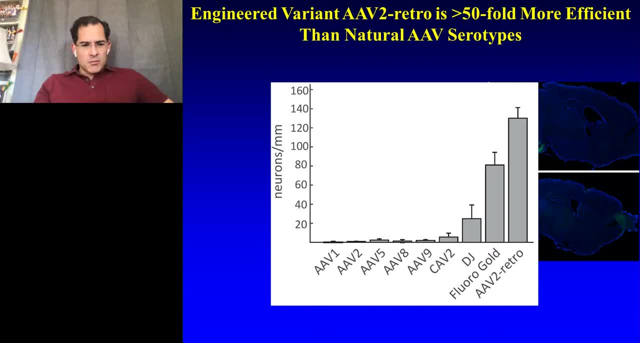 in the cortex expressing GFP. but it's not comparable to this variant, the AAV2 retro that we created, where you can see widespread transduction across those neurons. When we quantify the efficiency of delivery you can see that compared to AAV1,, 2,, 8, and 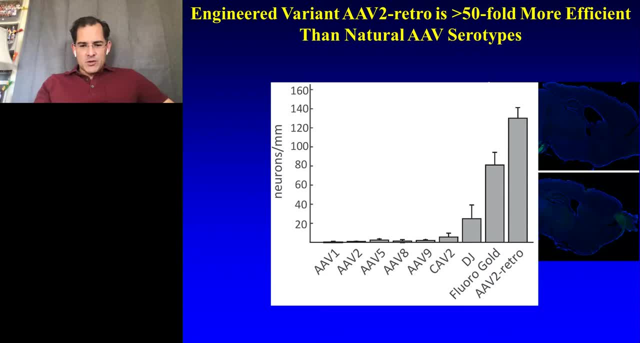 9,. we have 50 to 100-fold higher levels of retrograde transport, and it compares quite well to a number of other approaches for retrograde transport, including even this fluorescent dye in an organic molecule called fluorogold, which is being utilized for retrograde. 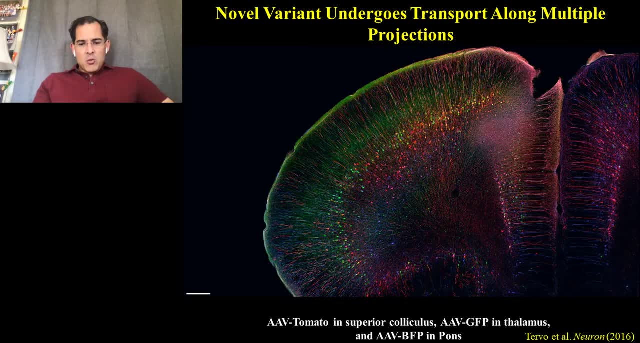 transport labeling. We then wanted to see strategically with a couple of different injections, how we could maximize spread across the brain and you can see here if we do three different injections with three different AAVs of three different colors- red, green and blue- into the superior. 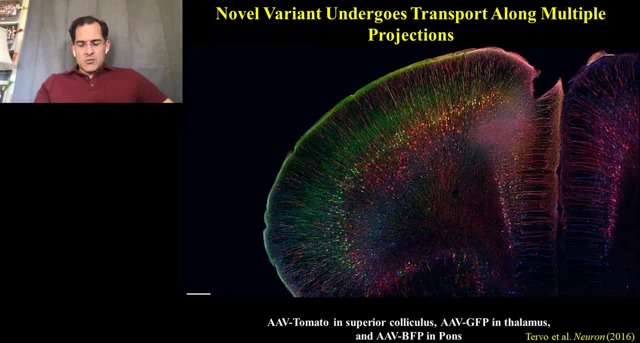 colliculus, thalamus and pons respectively. just these three focal injections gets you widespread expression across large volumes inside the brain, And we've since utilized this to affect genome editing within the brain as described in that article in the bottom right-hand side. 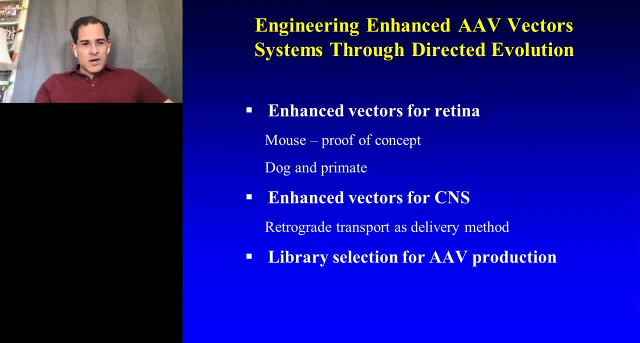 So I'd like to move on quickly to the final chapter of the work I wanted to describe to you today, which is going to be some work that carries on. So I'm going to go ahead and get started. So I'm going to go ahead and get started. 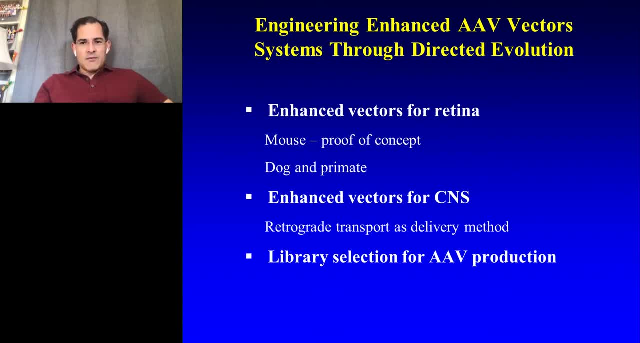 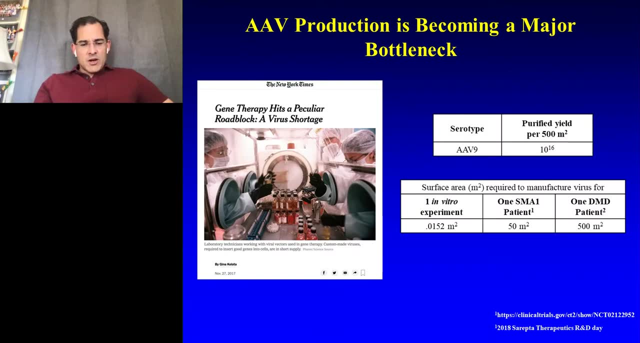 It carries on the same concept of solving problems through libraries and evolution, but now applies it towards a different problem, which is AAV production. So there's been, as gene therapy has been increasingly successful, there's been a bottleneck within the field related to AAV manufacturing, as shown here in this relatively old article. 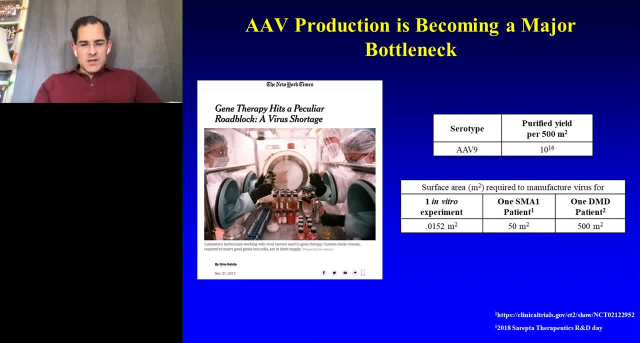 from the New York Times And this problem is illustrated here. So AAV serotype 9, which is the serotype that's used for that FDA-approved product to be able to treat spinal muscular atrophy. So from around a 500-meter-square bioreactor you can create on the order of 10 to the 16. 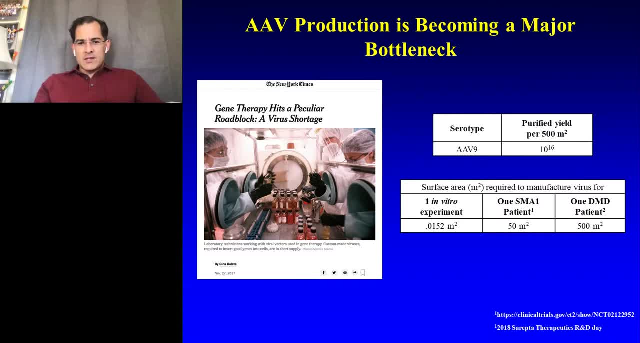 viral particles, So you can then translate in this into how much surface area you need to be able to treat individual patients who are suffering from certain conditions. So in the middle here we have one SMA patient and they typically treat this is Novartis. 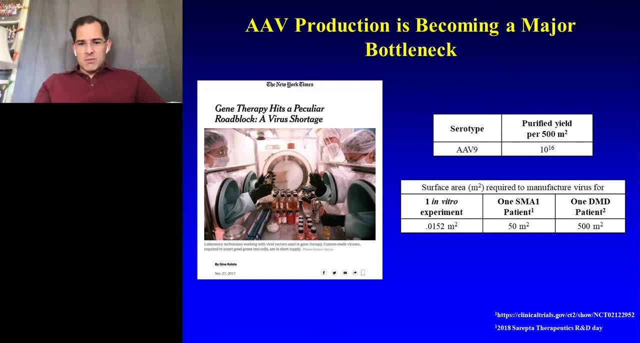 ovexus. They treat patients typically on the order of weeks of life. So they're treating young, young patients Just postnatally And as a result, you don't need as much virus because simply you know young patients aren't. 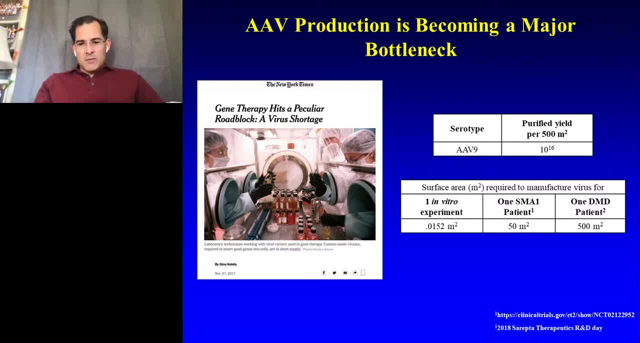 as big yet. So even so, you need around 50 square meters to treat one patient, And AAV 9 is also in clinical trials to be able to treat Duchenne muscular dystrophy, And in that case you need 500 meters squared. 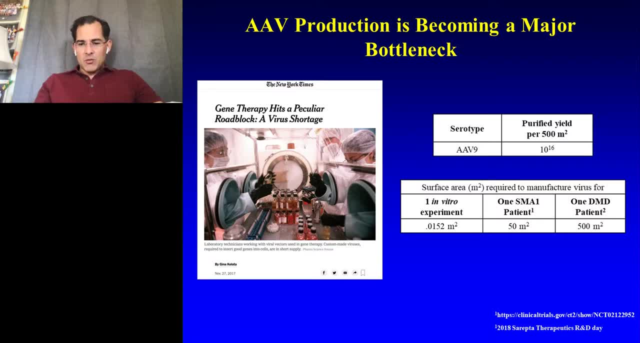 In other words, in some cases a single manufacturing run per DMD patient treated. So how does this translate to the incident and prevalent populations? You need around 200.. You need around 20,000 meters squared to treat the annual incidence of a spinal muscular. 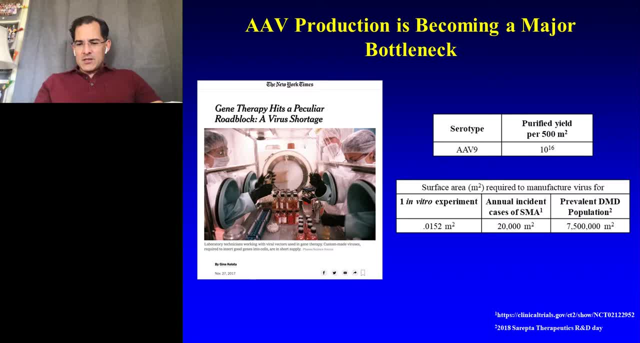 atrophy type one, and you need around seven and a half million square meters to be able to treat the prevalent Duchenne muscular dystrophy population. So this is actually hundreds of around the order of a thousand soccer ball fields worth of surface area. So they're quite simply it's going to be challenging to have enough manufacturing capacity. 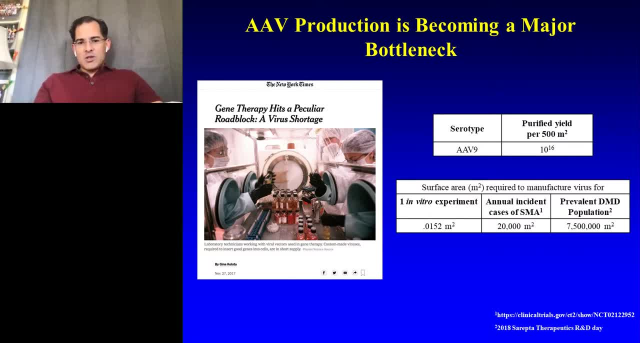 to treat these conditions. So one way in which you could ease the manufacturing capacity. So one way in which you could ease the manufacturing capacity. The other way in which you could ease the manufacturing burden is by creating an AAV that's much more targeted and efficient at being able to reach a tissue. 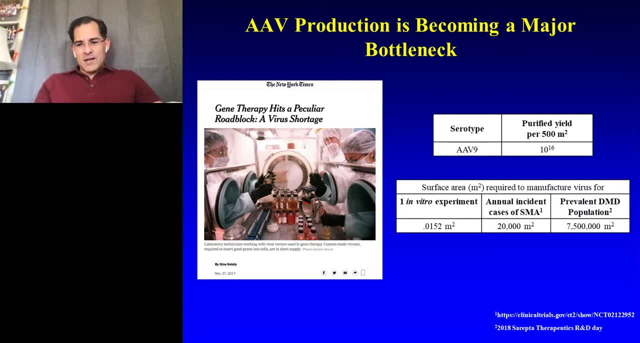 So let's say you created a directed evolution AAV that's a hundred fold better at getting there. Well, that's going to alleviate the manufacturing burden. But another way in which you could do it is to actually engineer the manufacturing cells to pump out more AAV. 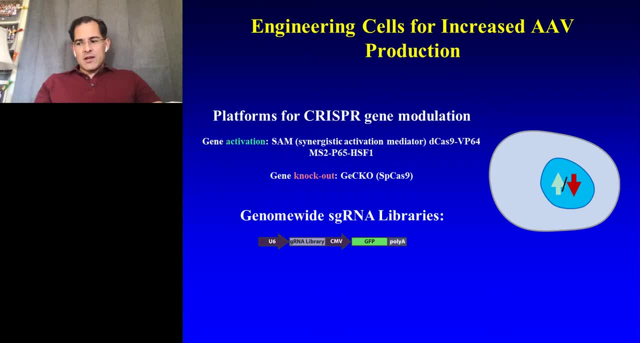 And we begin to do that using a that has an active nuclease and using a guide RNA. 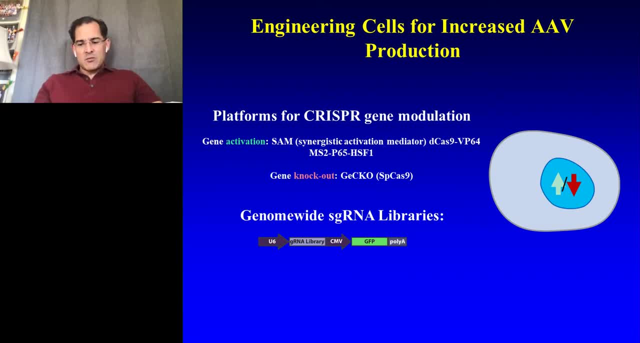 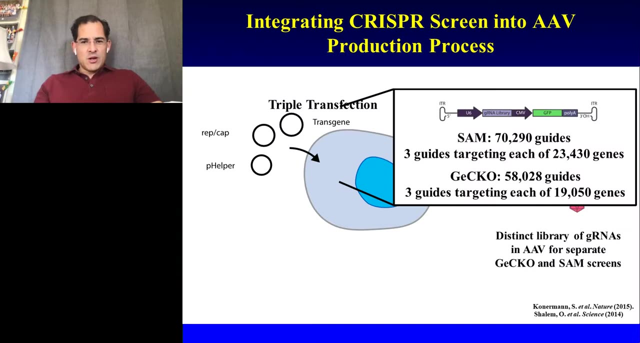 target that Cas9 towards, let's say, the first exon of every gene within the human genome and generate genome-wide knockout libraries. And so these guide RNA libraries are what direct these different systems, either a transcriptional activator or a knockout system, towards particular regions within the genome. 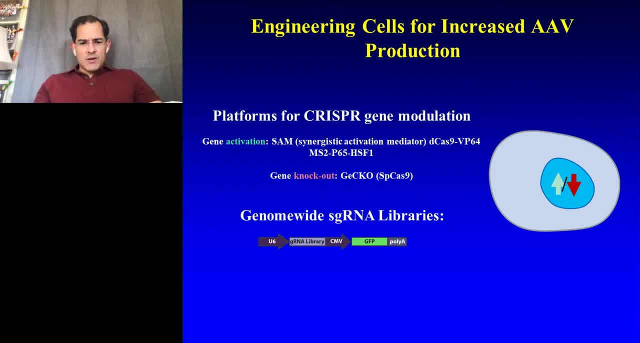 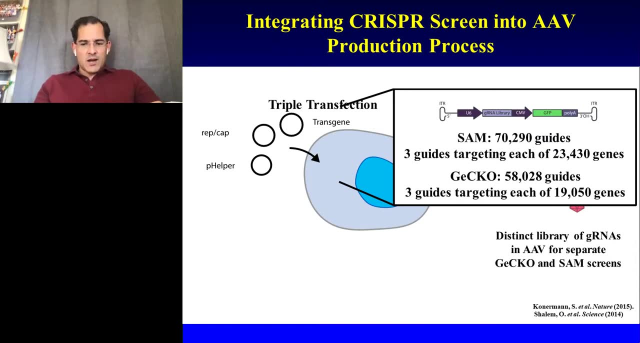 So we ended up embedding these guide libraries into AAV vectors so that we could select for guides or specifically for genes whose overexpression or whose knockout could increase AAV production. And we did this within 293 cells, which is the dominant manufacturing cell line. 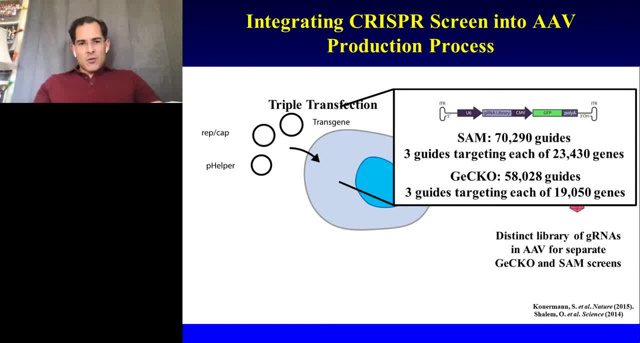 to produce AAVs. So the rationale for this was that, just like we'd anticipate that, nature has never evolutionarily rewarded in an AAV for the reach of photoreceptor on inside, deep inside the eye. you know, it's just, it's not part of the AAV. 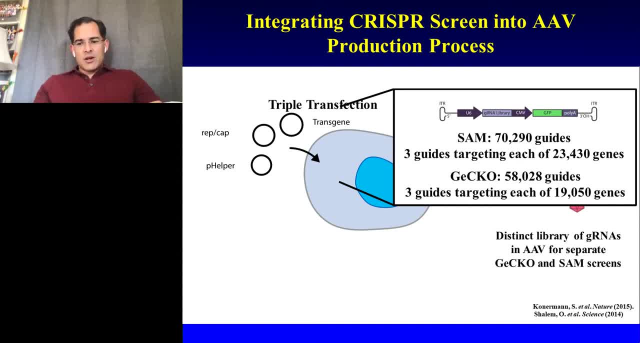 it's part of the AAV life cycle. Likely, nature has never evolutionarily rewarded a 293 cell, which is a transformed cell line that was derived from embryonic kidney. human embryonic kidney is never evolutionarily rewarded for the ability to pump out AAV. 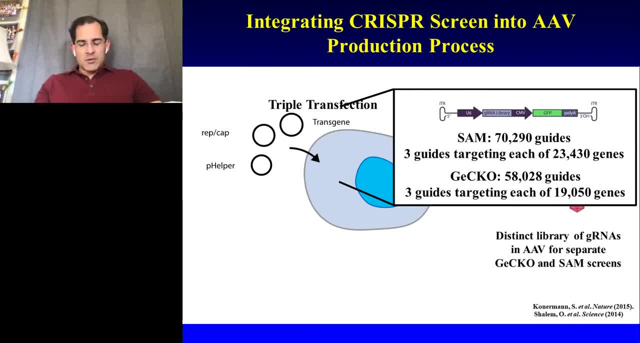 So it was the opportunity to engineer the cell line to be able to better do that. So the way that we did this is that we created libraries of guide RNAs inside of AAV, where we cloned in all 70,000 guides present within this. 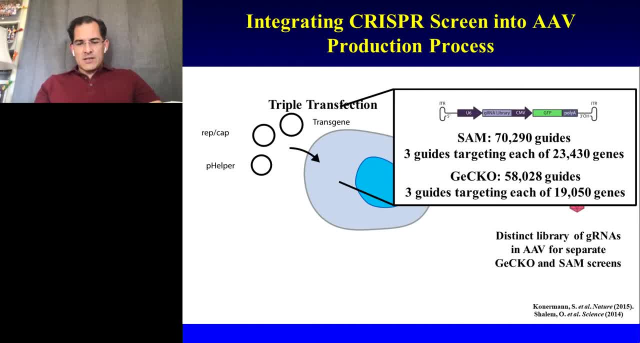 this traditional system, which contains the 70,000, contains three guides per gene for each of 23,000 genes within the human genome or the gecko. the knockout library contains three guides for each of 19,000 genes, so 58,000 guide library. 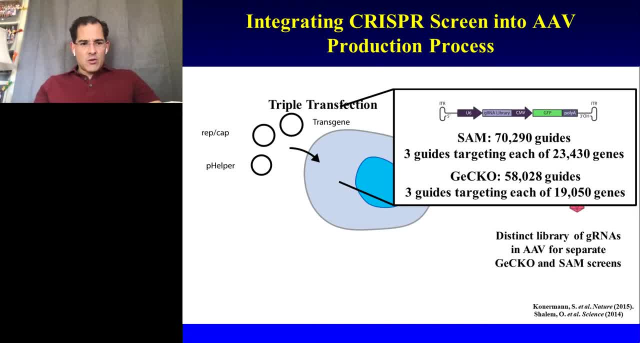 So we cloned those inside of AAV and packaged it along with the rep cap helper and an adenoviral helper so that we created libraries of AAV vectors where every single variant on the right-hand side has the same capsid gene, in this case. 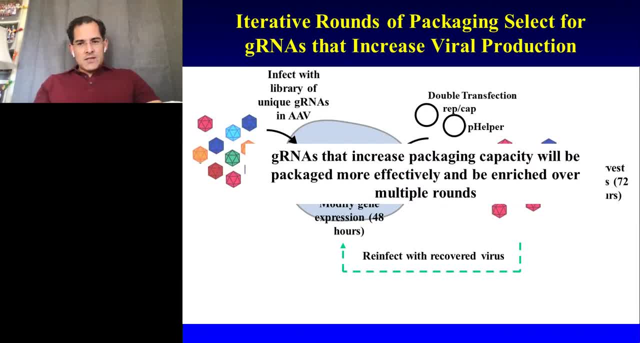 but contains a different guide RNA inside of it. We can then take these and infect it, infect cells with them at a low ratio of virus to cell. So each cell took up only one virus and, as a result, expresses only one guide RNA. 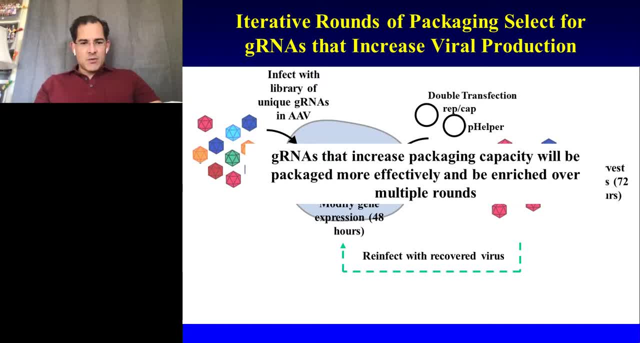 And these cells now have the CRISPR-Cas system, which can take the guides and either overexpress or knock out a particular gene, depending upon the nature of the AAV library. So we then gave this cell around 48 hours to perturb gene expression. 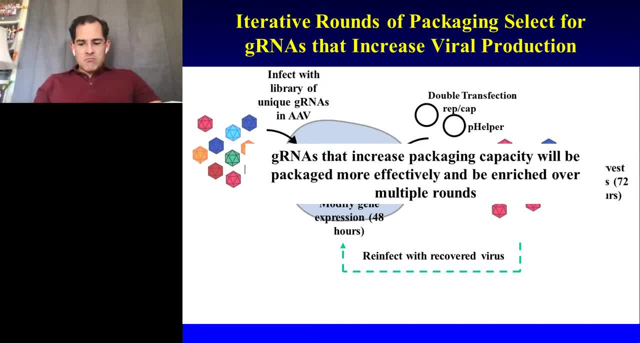 through that overexpression or that knockout and then transfected in the helpers so that we could then use that cell to manufacture AAV. And the logic is that if a particular overexpression of a given gene in the human genome or a knockout of a given gene in the human genome 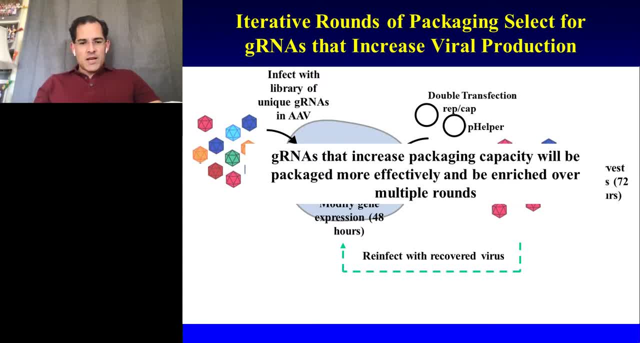 ended up changing the cell in such a way that it could better produce AAV, then that cell is gonna pump out more AAV. And just to remind you that AAV genome is gonna inside of it, The barcode, the information that tells us. 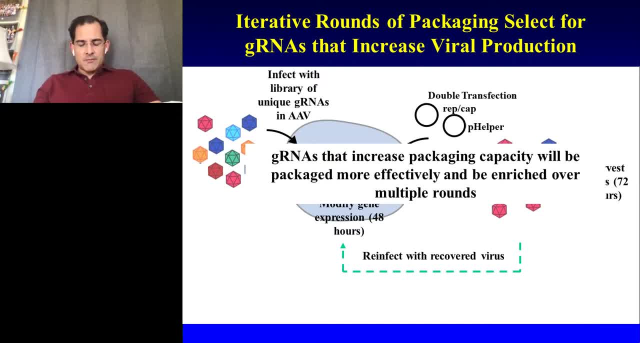 which gene perturbation resulted in the better production of AAV. So we can then harvest that library, use it to reinfect the cells, repackage And, as time goes on, the AAV variants, that or the guide RNAs, if you will, inside those AAVs. 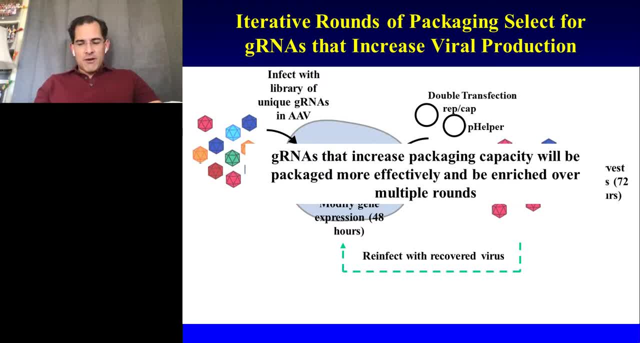 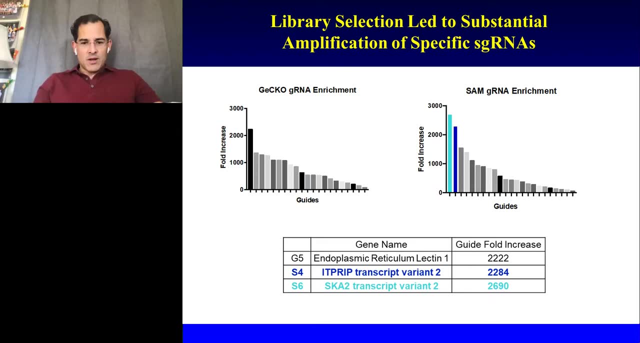 that results in better packaging are gonna get exponentially amplified within the population. And at the end we can then do sequencing, next-gen Illumina sequencing to sequence the guides and tell us which genes whose perturbation would result in an increase in AAV production. 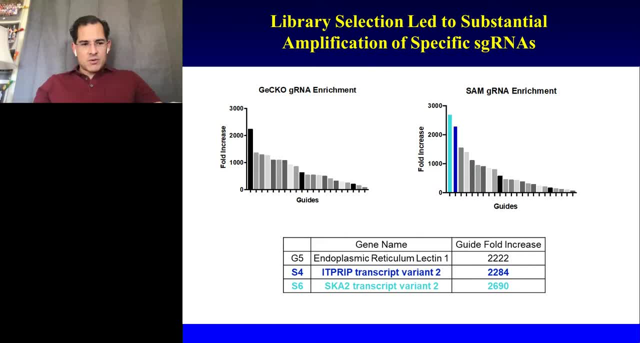 So we have a number of different hits and two particularly interesting hits emerged from the overexpression library. One is called ITPRIP, which is an inositol triphosphate receptor interacting protein. So this modulates calcium release inside of cells in response to signals that release. 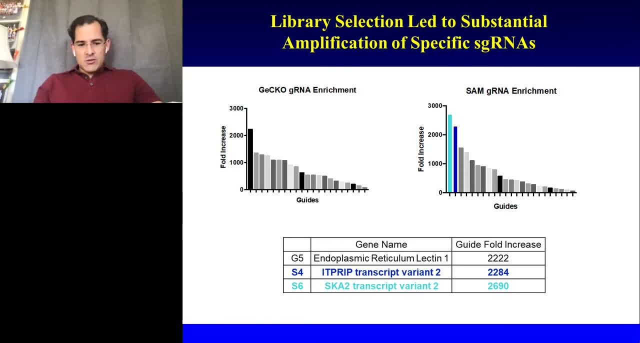 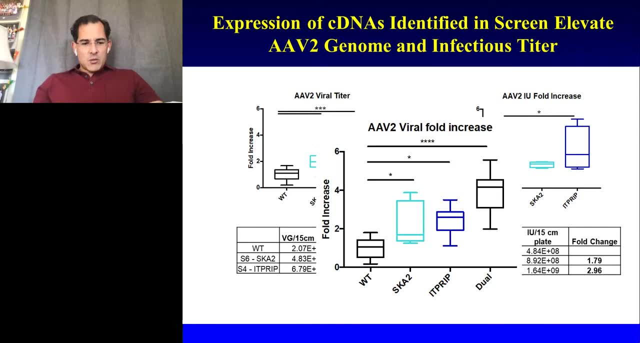 that result in ITP production, And Scott two, two spindle and kinetic core associated protein type two which is involved. So we took cells, 293 cells, and overexpressed these two proteins, initially by overexpressing the guide and Cas9 system. 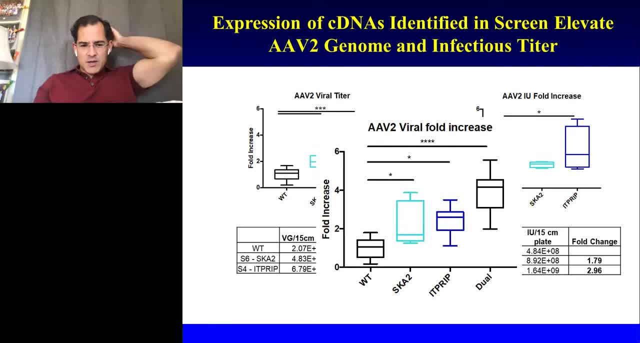 And then we did encoding these proteins and overexpressing them inside of cells And we found out that upon overexpression of these proteins, we get around a two to three fold increase a through production from these cells, And this is both at the level of vector genomes produced. 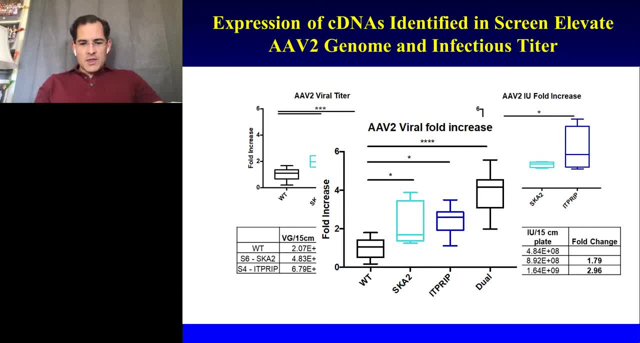 as well as infectious units produced, And furthermore, there was the possibility that these two genes could be acting independently within those cells and therefore by combining them we could get synergistic increases. And we see that upon overexpressing both cells, we get around a four to five fold increase. 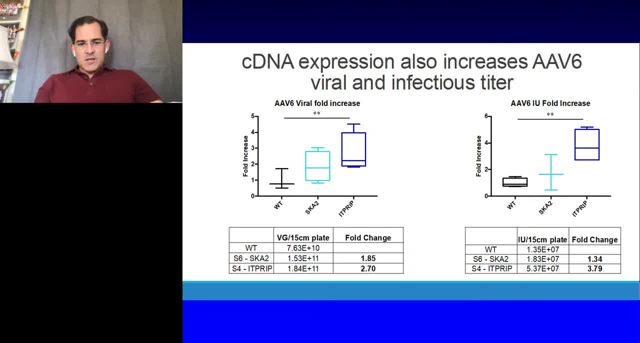 in vector production And, furthermore, this was not limited to AAV2, but extended to other AAV stereotypes, such as AAV6,, which is notorious for being a particularly difficult to produce, And we see a two to four, around a three to four increase. 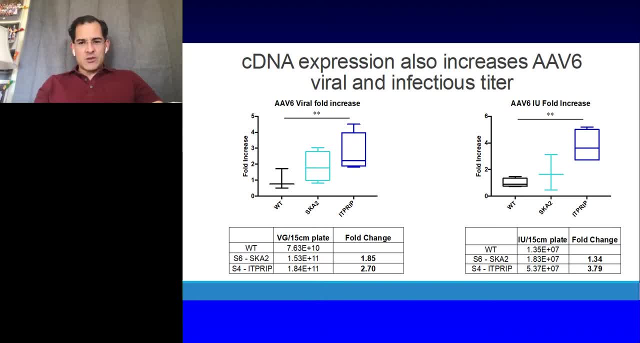 in both viral titer- genome titer- as well as infectious unit titer. So we have since this test to getting mechanisms by which overexpression of these genes ends up resulting in better AAV production, And we're seeing evidence that these genes. 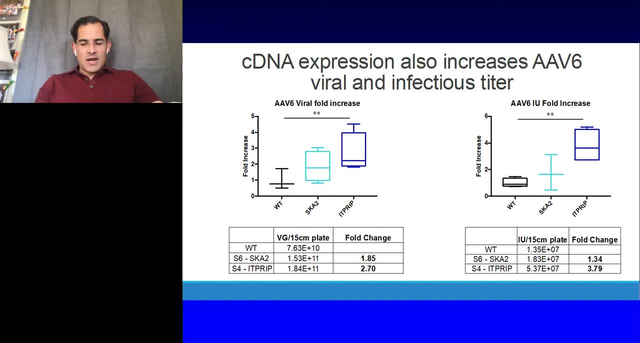 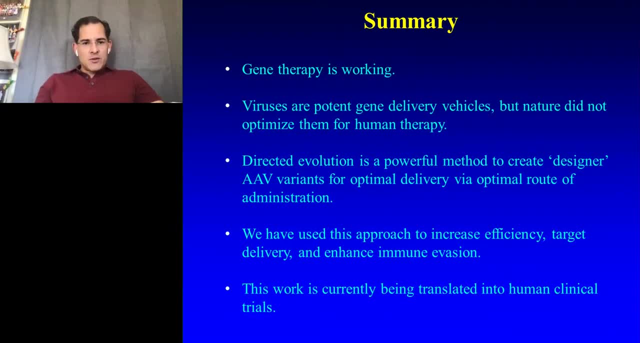 actually perturb cell cycle in a way that is advantageous for AAV production, And we look forward to going into detail into that mechanism soon. But I'd like to close now with a few bullet points from the work that I have presented. The first is that gene therapy is working. 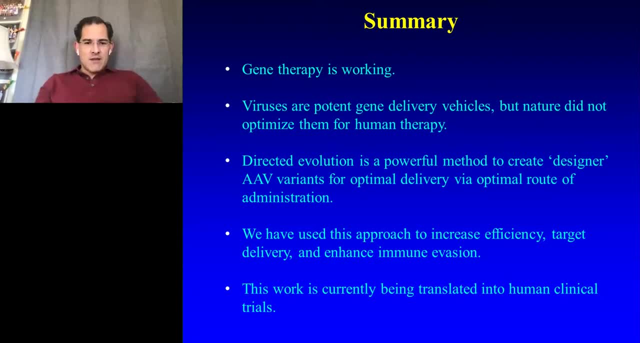 In addition, recombinant safe viruses like AAV can represent very potent therapeutic pharmaceutical gene delivery vehicles, But of course, nature didn't optimize them for use in human therapies And therefore it's up to us to re-optimize these viruses to be safe, effective, efficient therapies. 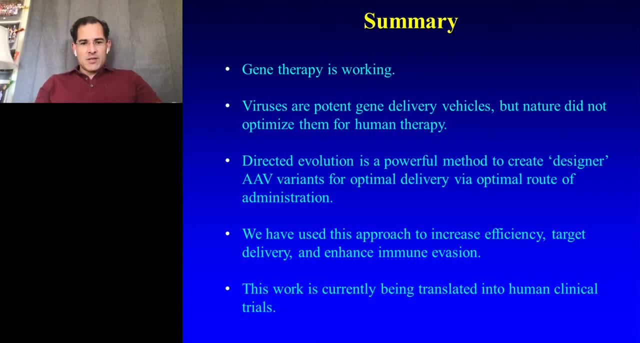 So these particles are very complex, complex products of millions of years of evolution, And it's very difficult to rationally engineer changes into them. However, directed evolution ends up being a very powerful search algorithm where we can search billions of potential viral sequences to be able to isolate the variants that 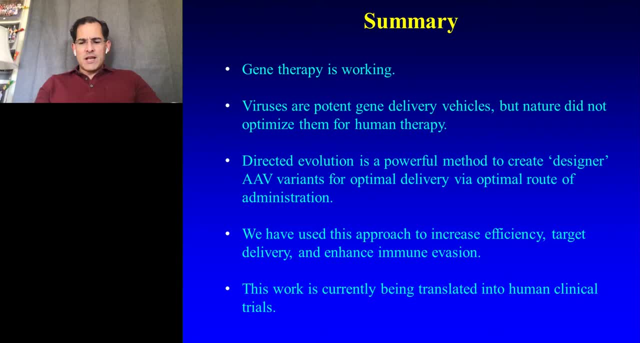 have highly optimized properties for delivery in principle to any cell or tissue target through an optimal route of administration, And we use this approach to create AAVs that are highly efficient, can target delivery or in work that I didn't talk about today. 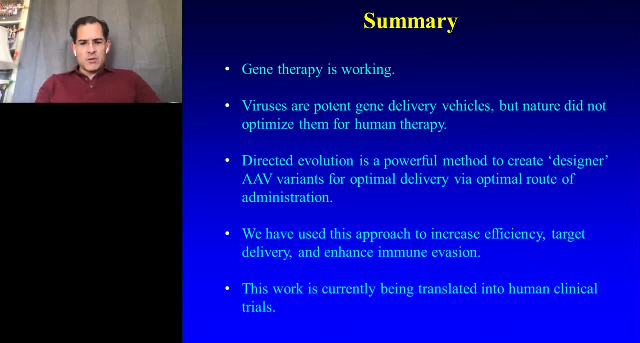 It can also get past that pre-existing antibody problem within the human population. So one of the AAV variants we've created has already been in the clinic for almost a year and a half, And several additional variants are going to be entering into the clinic this year. 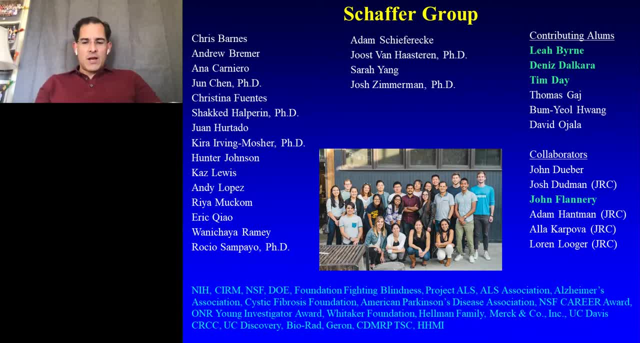 So I'd like to acknowledge the people who actually did the work. The work within the retina was the product. This is mouse retina, the product of Leah Byrne, Denise Dolcara and Tim Day, in collaboration with John Flannery at UC Berkeley. 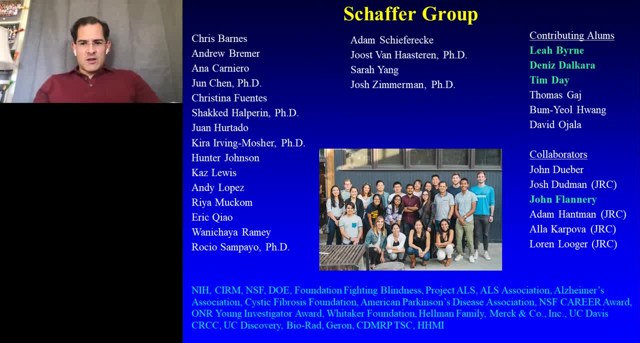 The work in the dog retina was the product Again Leah Byrne at UC Berkeley and John Flannery in collaboration with Welling Beltran University of Pennsylvania. The work in the non-human primate retina came out of 4D molecular therapeutics.